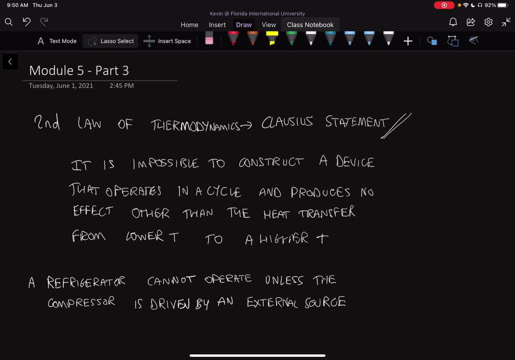 In part 3 of module 5, we're going to continue our discussion of the second law of thermodynamics and specifically the Clausius statement, And then we're going to go into looking at reversible processes and irreversible processes and how we can apply some equations to essentially a perfect 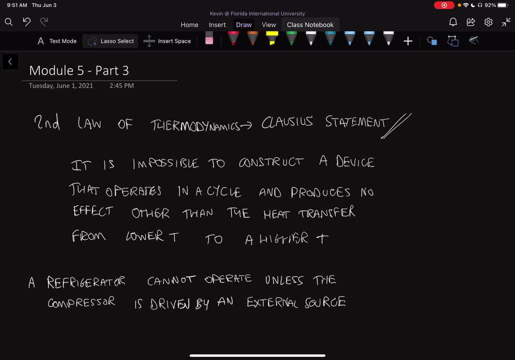 cycle. So to start with, we're going to read out the Clausius statement and make some comments about it. So the Clausius statement says that it is impossible to construct a device that operates in a cycle and produces no effect other than the heat transfer from low temperature to. 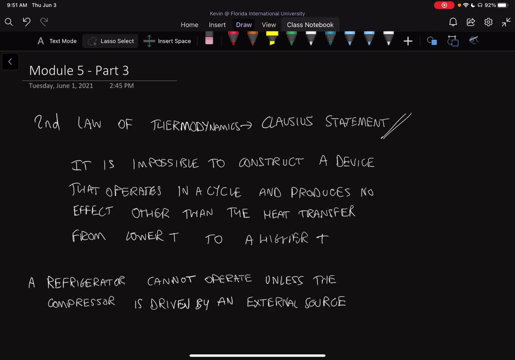 higher temperature. And what this really means is just: it states that a refrigerator cannot operate unless the compressor is driven by an external power source or a motor. Okay, if there is no motor, then the compressor is not able to operate. If there is no motor, we can't get our heat transfer to go from low temperature to high. 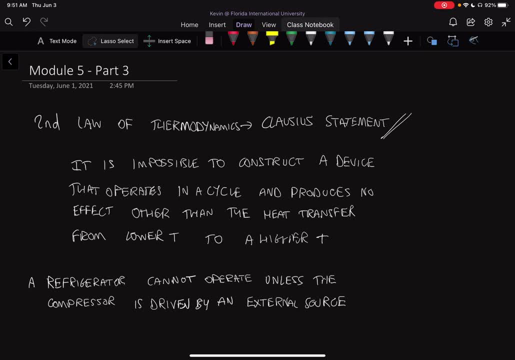 temperature. Okay, usually we always know: if we have a hot temperature fluid mixed with a cold temperature fluid, the temperature is going to go from hot to cold. Now the only way for us to make it go from lower temperature to higher temperature, from an experimental point of view, is to add: 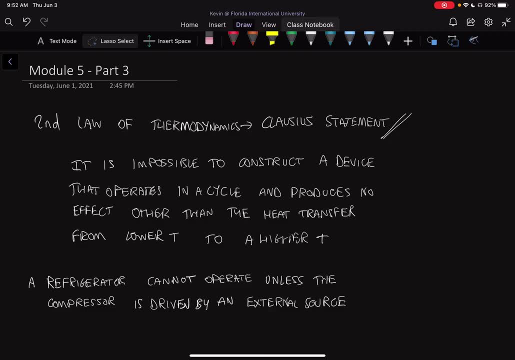 some sort of motor Or some sort of power source that is external. Okay, now this and the Kelvin-Planck statement. So the Kelvin-Planck statement said that it is impossible for any device that operates on a cycle to receive heat from a single reservoir and produce a net amount of work. So that was more. 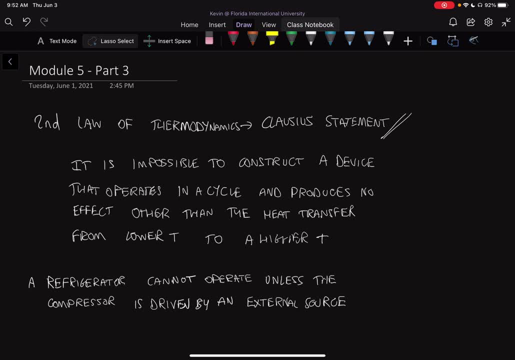 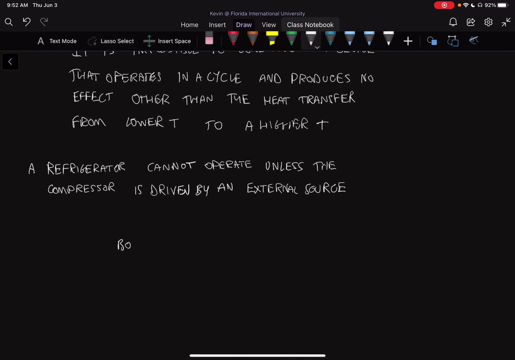 to do with our power plant, for example, or our heat engine. Both statements we can say are impossibilities. Okay, so we can say that, both statements so, the Clausius and the Kelvin-Planck which we had looked at earlier. 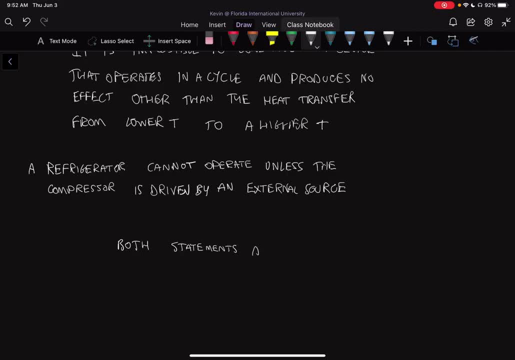 both statements are negative, meaning that they say that the process is impossible, So they're not really proven. Okay, we can't prove an impossibility, because we can always have it happen, We don't know. But the reason here is that it's 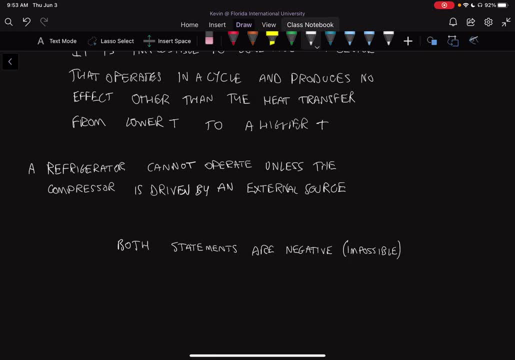 impossible because it's never been proven experimentally. We haven't been able to prove experimentally that we can transfer heat from lower temperature to higher temperature without doing any work, for example. So the second law we can say is based on experiments, Experimental evidence. 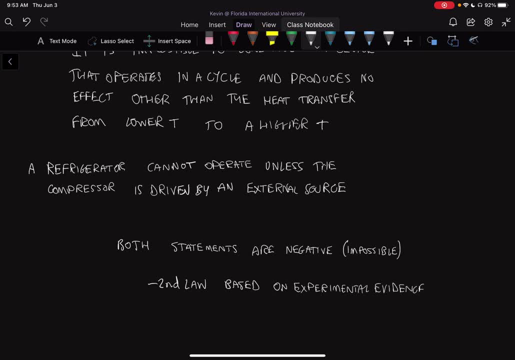 And the experimental evidence points towards these two impossivities. Okay, so we cannot prove otherwise. we cannot prove a negative, but we cannot prove that we have experimental evidence of something going from a lower temperature to a higher temperature. So the second law is not a law. that is a typical law where we can prove it with experiments. 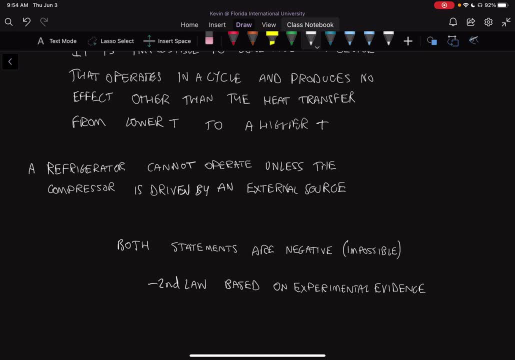 In this case, what we're doing is we're saying, by experiments, it is impossible for this to happen. We've never seen it happen, Therefore, it is impossible. Okay, So now let's talk a little bit about what a reversible and irreversible process is, because it's going to be important for our discussion of an ideal cycle, essentially. 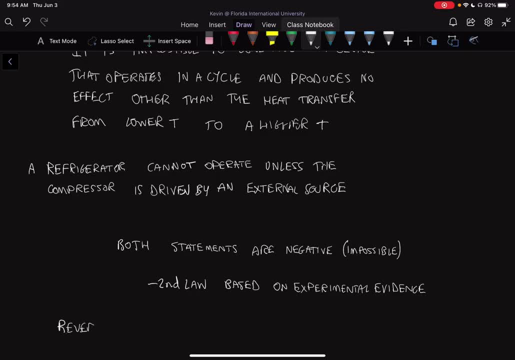 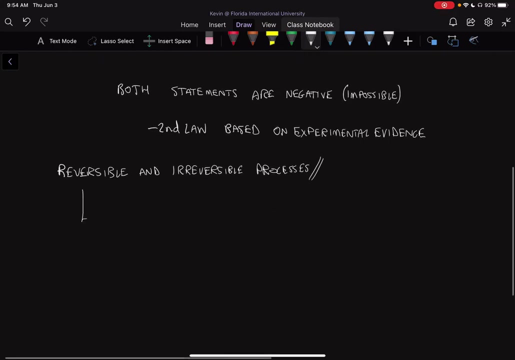 So we're going to be talking about reversible and irreversible processes, And so you might have seen this before, but a reversible process is essentially a process that can be reverted without leaving any trace in the surroundings. So it's a process that can be reverted without leaving any trace in the surroundings. 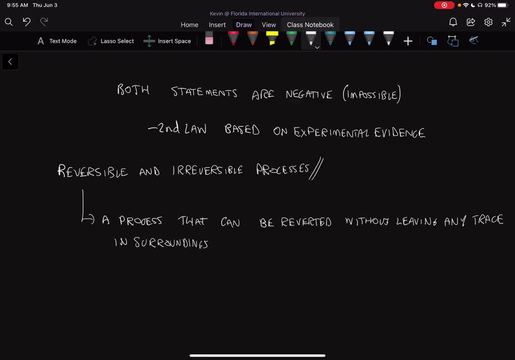 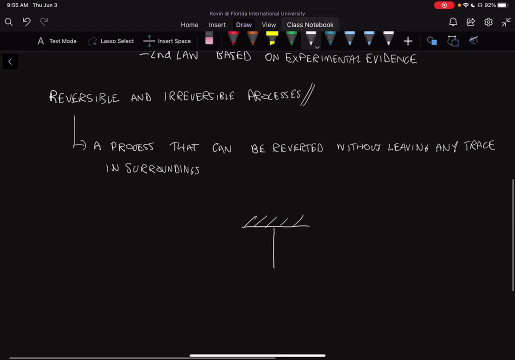 So, for example, an example of a reversible process would be a process like this: We would have a pendulum hanging from a string and this pendulum would be swung up and down. And if this pendulum, If this pendulum is frictionless- okay, if we assume that it's frictionless- this would be a reversible process, because our pendulum would move from left to right, keep moving from left to right without any friction, and it would be perpetual. 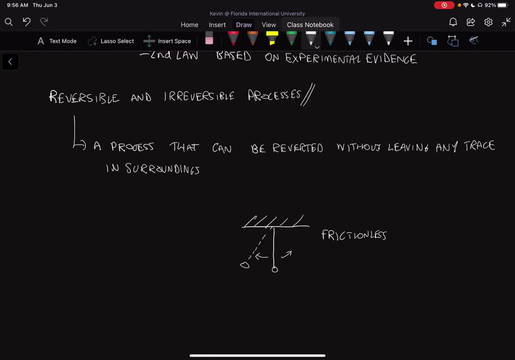 It would happen throughout time. It would never slow down if we give it that initial energy to move. essentially Okay. So that's an example of Of a reversible process And this reversible process can be called. We can say that it is an idealized process. 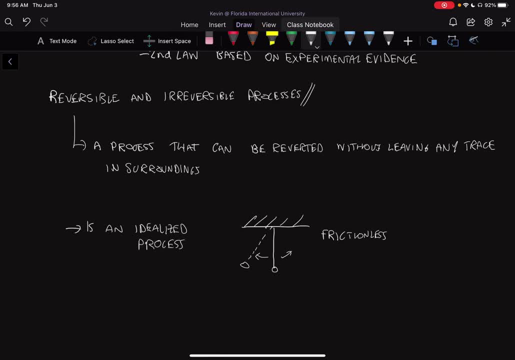 So in real life, reversible processes don't really exist. Okay, We never have a fully reversible process. If we have some friction in a pendulum over time And because of wind resistance, for example, over time the pendulum will slow down more and more and more and some energy will be transferred to the surroundings. 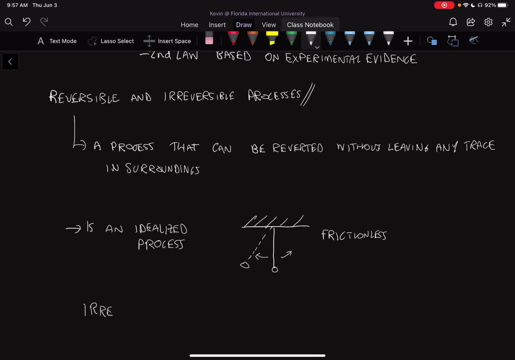 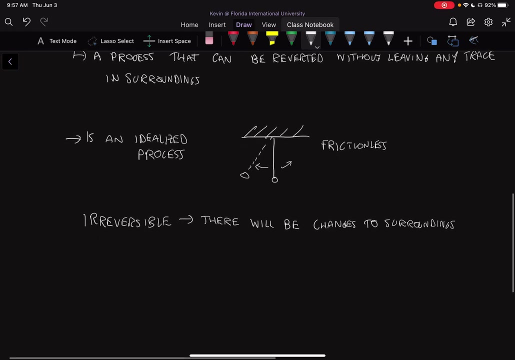 And that's what an irreversible process is right. So an irreversible process is just a process where there will be changes to the surroundings. Okay, And we've said that reversible process is something that does not occur in nature, So we can go back to reversible. 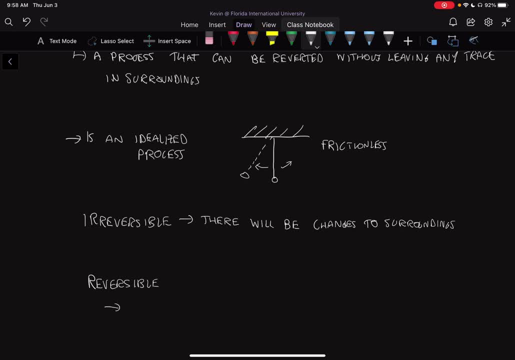 and say that reversible processes, Reversible processes, Reversible processes are a limit to or a limit for reversible processes, for irreversible processes, sorry, okay, so they are essentially the theoretical limit where an irreversible process can reach. so if we have very, very, very little friction, we're going to get very close to a reversible process. okay, in the 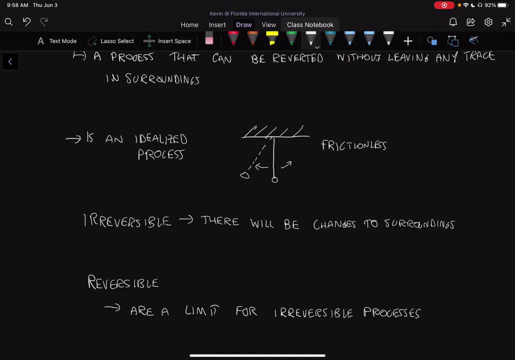 case of our pendulum, if we're nearly frictionless, it's going to take a very long time to lose that energy and to lose that momentum in our pendulum. now it's also a way of a reversible process, is also a way to compete with the pendulum. in the case of a pendulum, it's also a way to compete. 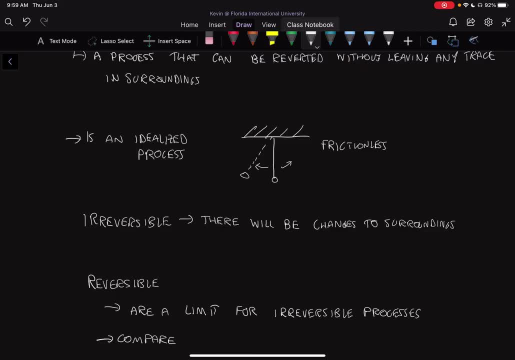 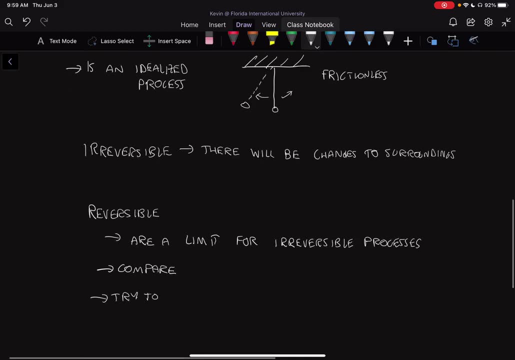 essentially what we have between our real process and perfection. okay, it's a way that we can use to try to reach perfection, to reach perfection in our system or to set a goal. so, as engineers, we always want to try and set a goal to lose as much energy to the surroundings as possible. 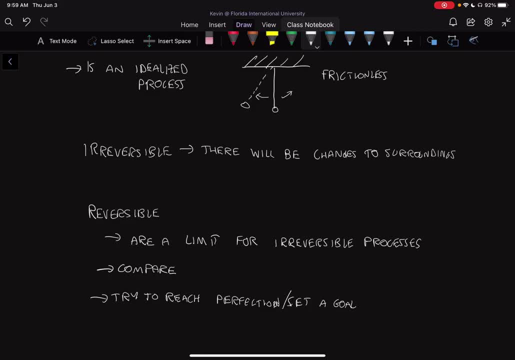 and so that means that we're trying to set a goal to get as close as possible to reversible process. now, this is not always possible, but what is nice about a reversible process is, if we know this, this is our theoretical limit. it actually makes it easier to analyze. 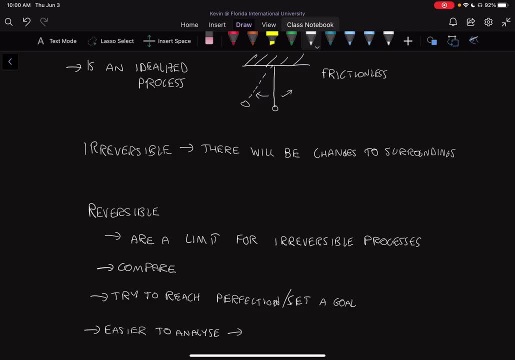 compared to a in a reversible process where there could be friction, heat transfer or some other types of loss of energy, where it's a lot harder to solve for a problem theoretically okay. so it's easier to analyze because it can be solved completely theoretically and then we can measure our difference between our theoretical and our practical. 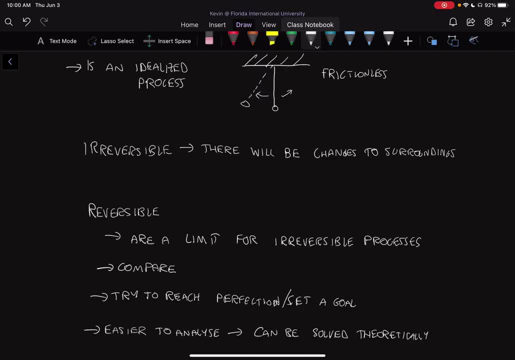 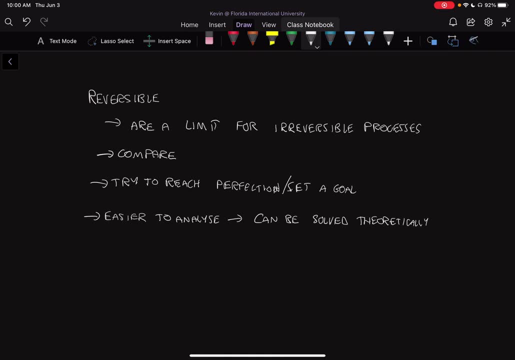 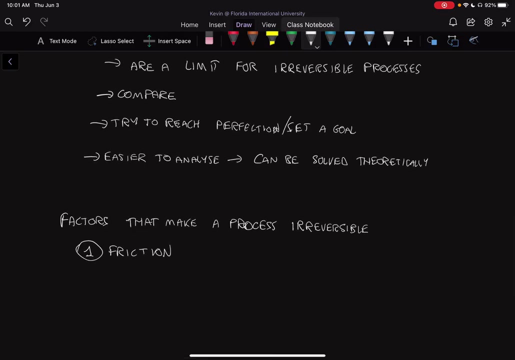 by doing some experimentation, essentially. so looking back at irreversible now. so the other type of process, the process where we have some losses, what are some factors that make the process a risk, like a process irreversible? so we've already talked about a few, but the first one we can talk about is friction. 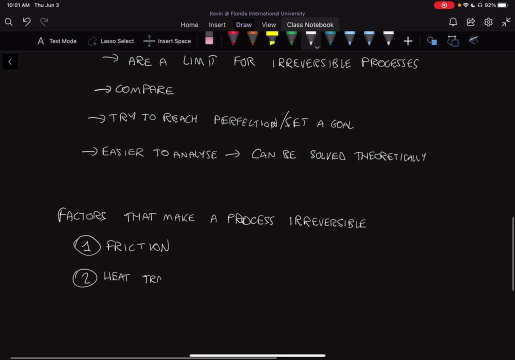 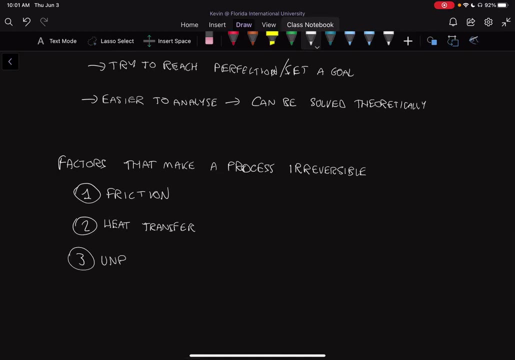 also have heat transfer. if we have heat transfer from our system to the outside, we are going to have an irreversible process. we sometimes can't get the heat transfer back in. and three, it is what is called unrestrained expansion, and we'll look at that in a minute. so the first of an example with our, the first example, we 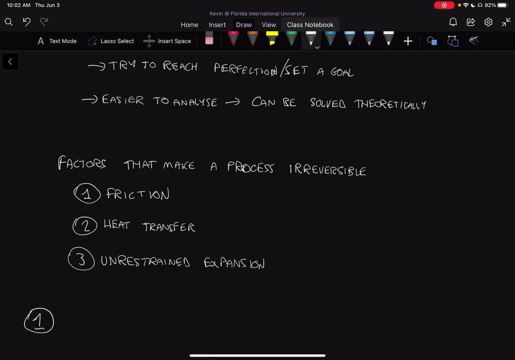 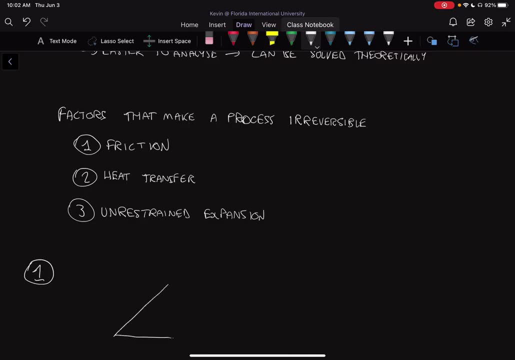 can have is for friction. so if we look at one, a typical example of friction is: let's say, we have an incline and on this incline at the top we have a pulley and we have a block here. block one is being pulled down by another block two, it's being pulled down by gravity. 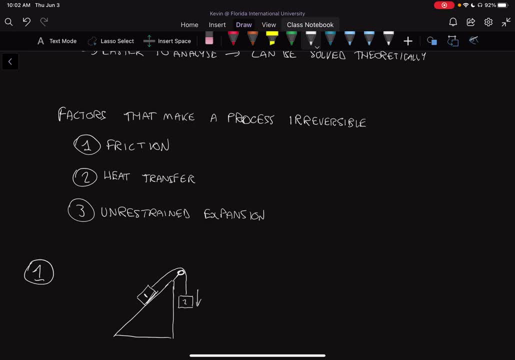 and so this block is going to go up this way, okay, and because of the friction, what's going to happen? we're going to have an increase in temperature. so, due to friction, so if, in in first instance, we go up with our block, with number one, due to friction, our block. 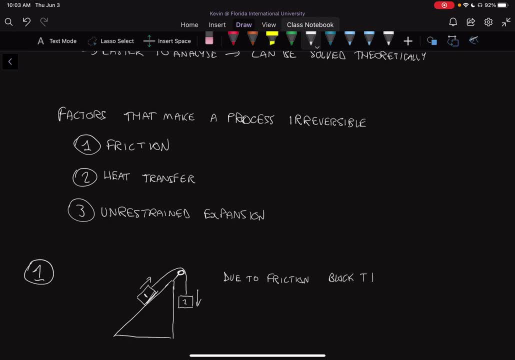 temperature is going to go up and in a second instance, if we now decide, let's bring it back to its original position. so let's bring two back up and one back down, we're going to have even more temperature because of the friction. so we started our process with a block, for example at 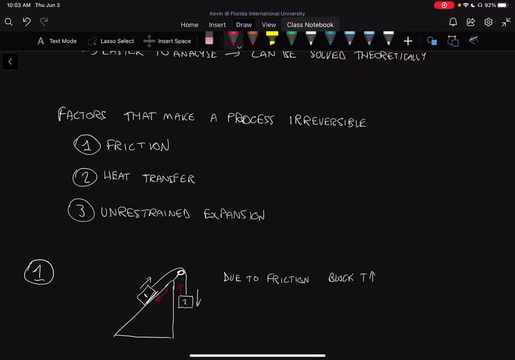 20 degrees. it went up a little bit. now the block was at 25 degrees and then it went down again and the block was once again at 28 degrees or 30 degrees. so it kept going up in temperature as the friction increased by the block moving. so we can't get back to our original state, which would require 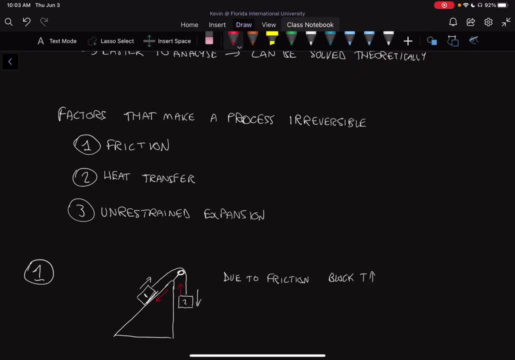 which would be a requirement for our reversible process. we need to get back to the same state as before. so that's an example of a process that is not reversible. we can't reverse the process and get some temperature out of the block okay, now. over time the temperature might go back down to 20 degrees. 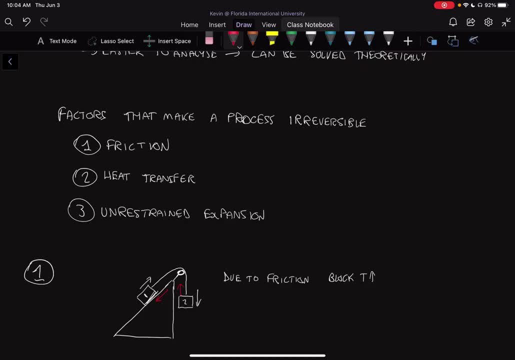 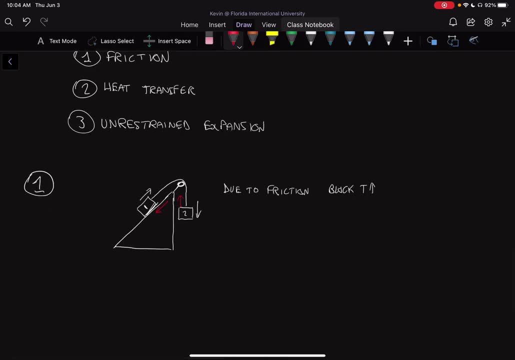 but now we've had some heat transfer out of our system. okay, for for number two, we can take the example of: let's say, we have a refrigerator and we refrigerate a soda. we decide that we refrigerate a soda in. we refrigerate a soda, okay, and our soda was for. 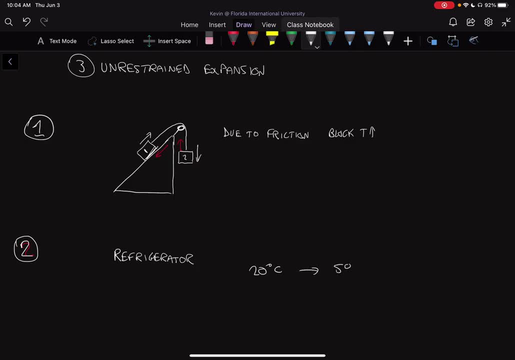 example, at 20 degrees celsius, and we refrigerate it and we bring it to five degrees celsius. okay, so heat is now transferred from the soda to to the refrigerator, to the refrigerator, and the soda is now at five degrees celsius. okay, so we have our can of sodas that's at five degrees celsius. we refrigerated it. now, let's say we now. 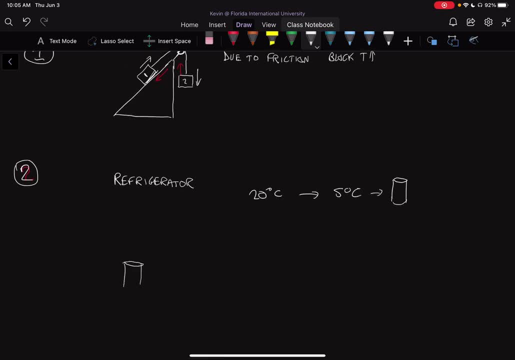 take the soda out and we put the soda in a room at 25 degrees celsius. so we put our five degree celsius soda in a room at 25 degrees celsius. now what happens is we have heat from the room is transferred to soda. we know that the heat goes into the soda. okay, we have some q in. 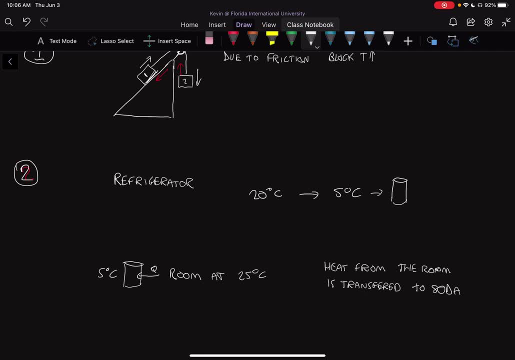 now, the only way to reverse the cycle is to refrigerate it again. so the only way for us to get our temperature back into the room at to 25 degrees and our soda back to five degrees would be to refrigerate it again. and if we refrigerate it, we require work input. 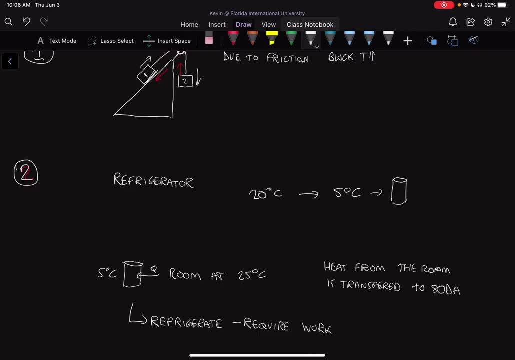 so we require some work in order to refrigerate it, to bring it back to temperature, so it's not a reversible cycle. so a soda that warms up in a room and then has to be refrigerated essentially releases heat to the environment and requires work. so we can't do it as a reversible. 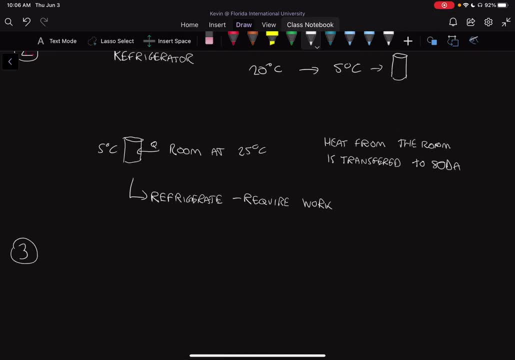 process. now number three, which is unrestrained expansion, can be explained through an example. that's pretty simple. so let's say we have, let's say we have a box here with some gas and we have a membrane. so this is a membrane and here we have a vacuum. 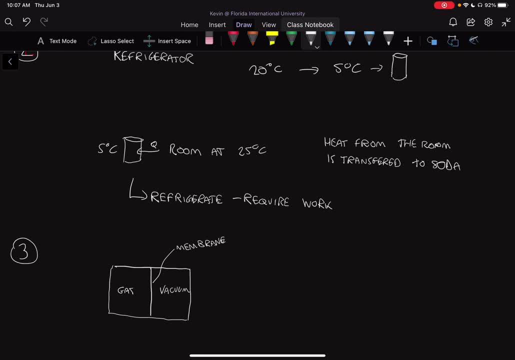 okay, so we have a gas here, initially on one side of the membrane, and then the other part of this volume that is, let's say, sealed completely. the other part of this volume is vacuum. now what happens if we take out the membrane? if we take out the membrane, the gas would expand. 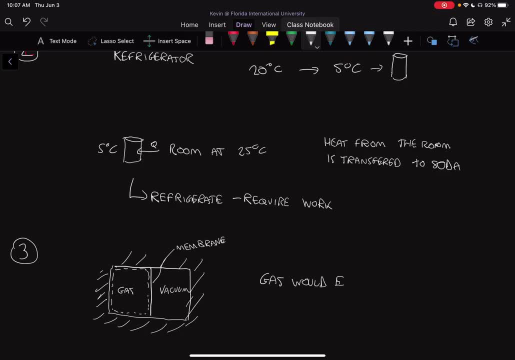 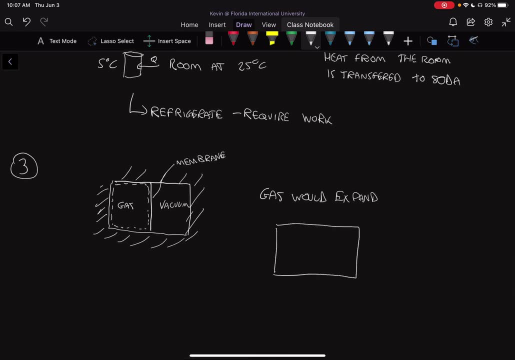 so we have a vacuum and we now have a system with gas everywhere. okay, so we go from a gas and vacuum to gas everywhere. now how do we get back to our original position? can we reverse this process? how would we reverse this process if we just add a membrane in a gas tank? it's just going to split the gas in two, so we 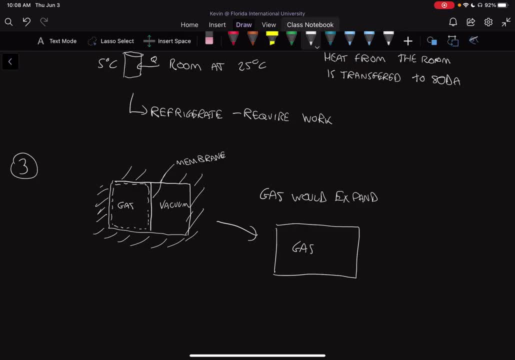 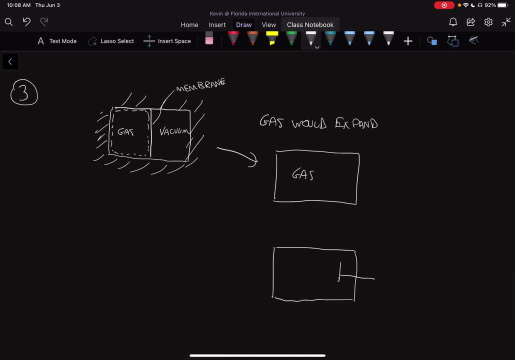 so the only way for us to get back to our original position is to essentially take our gas and compress it with some sort of piston and do some work in order to push it back. so, push the gas back to one side of the room, okay, so we would have to do some work, and that means that we don't have a reversible process. 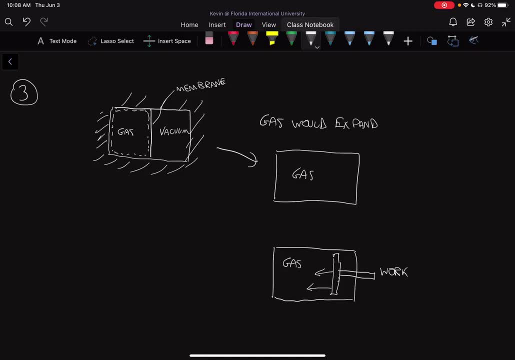 in one direction, we just had the gas expand, nothing, nothing had to be done. and on the way back, we have to do some work. so we clearly don't have a reversible process. okay, so this concept of a reversible and irreversible process is now going to be used to analyze some problems for 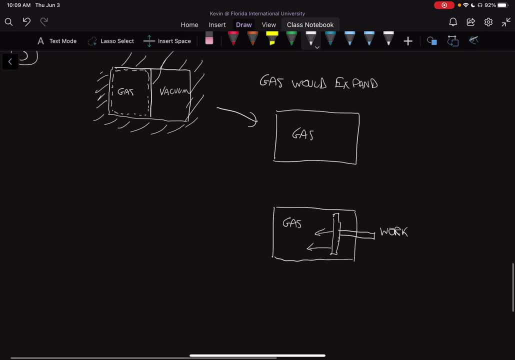 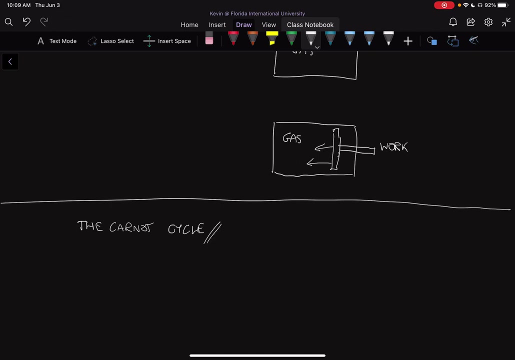 our heat engines and our refrigerators. so what we're gonna do is we're gonna study what is called as the Carnot cycle, and what the Carnot cycle is is essentially our most efficient heat engine. so it is a theoretical heat engine that operates at maximum efficiency, and it 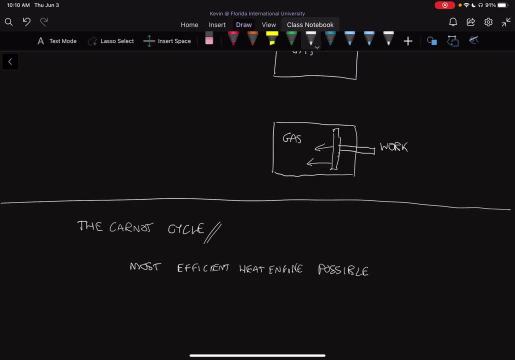 operates at maximum efficiency thanks to a theoretical assumption that we're gonna know that every cycle is essentially every process is essentially reversible within our system. so we're gonna make some assumptions and we're gonna write those assumptions down now. the first thing to note is that the most efficient heat engine possible does not have a thermal efficiency equal. 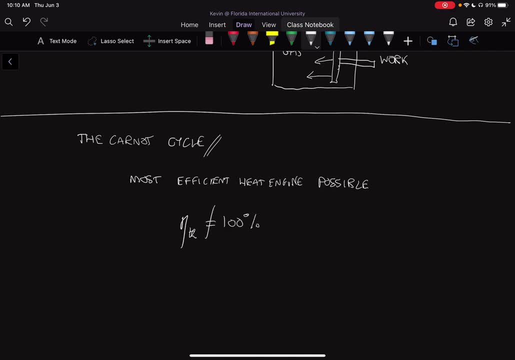 to 100%. it does not have a thermal efficiency equal to 100%. okay, that's really important to note and we'll see why. okay, so some of the assumptions we're gonna make. so we're going to assume that the heat engine, in this case, 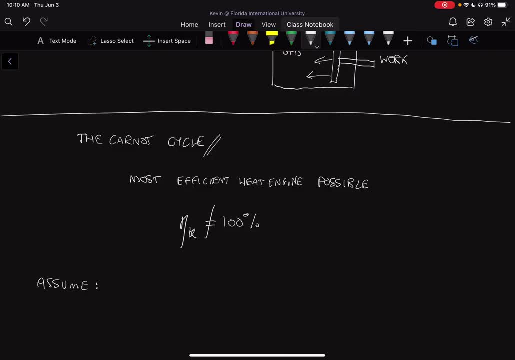 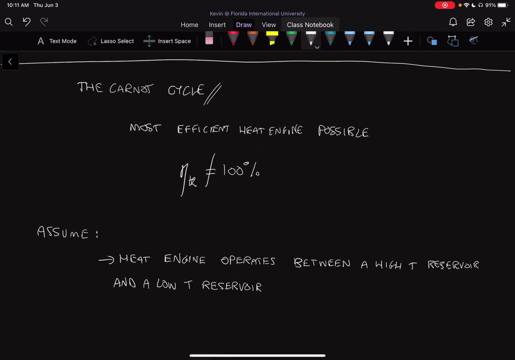 so in this Carnot cycle case, we're gonna make some assumptions, because it's a theoretical maximum engine, the best engine possible. we're gonna say that the heat engine operates between a high temperature reservoir, you, so we are going to have a constant temperature, regardless of Q, within our 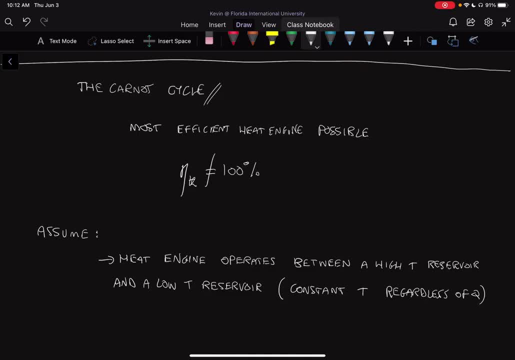 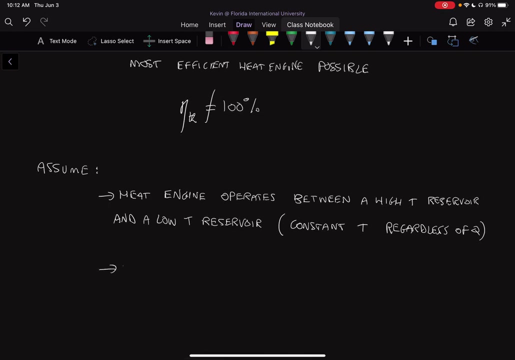 system in our high temperature reservoir and low temperature reservoir, and that means that the temperature that is used for the heat exchange is going to be constant. and it will make sense once we look at an example. okay, so the other assumptions that we can make is that it operates in a cycle in 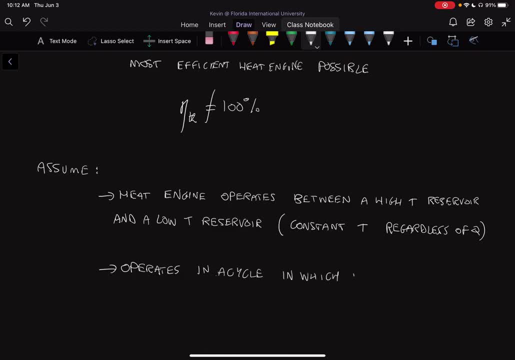 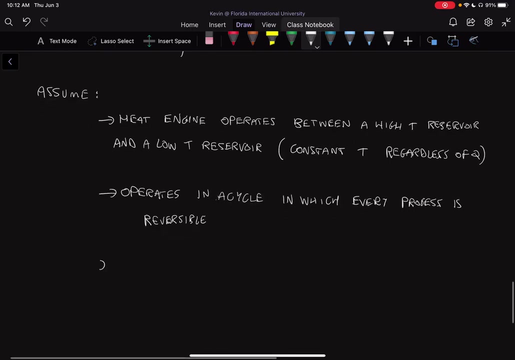 which every process is reversible. so every process within the cycle is reversible, okay, and that means in turn that the whole cycle is reversible. so that means we can switch a direction in our cycle and the cycle can be completely reversed. now, if a heat engine is completely reversed and is completely reversible, 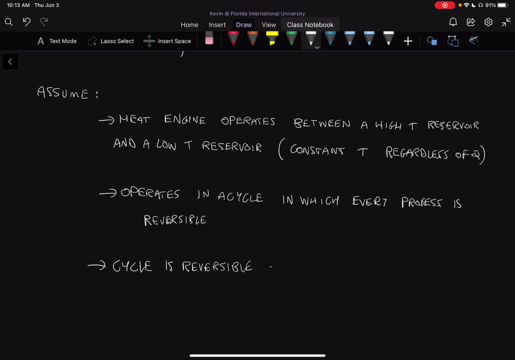 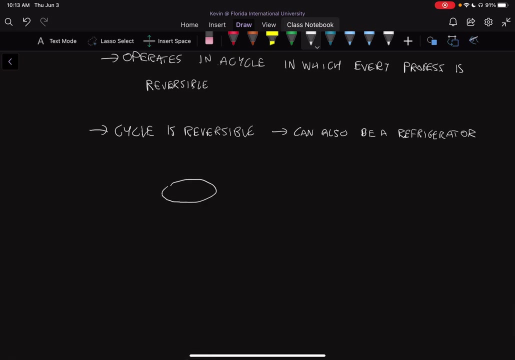 that means that it can also be a refrigerator. so that means that it can also be a refrigerator. so if we reverse everything in a heat engine and all the processes are reversible, that means that it can also be a refrigerator. okay, so it looks. it would look something like this: so we have once again, like before, we have our high temperature. 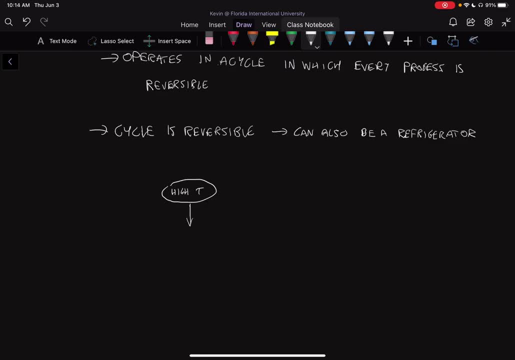 reservoir at the top bringing in some heat into our heat engine and there's some heat out to a low temperature reservoir and we have some work out, some work net. okay, if we can reverse all the processes, it means that we can essentially have something like this as well, with now work in. 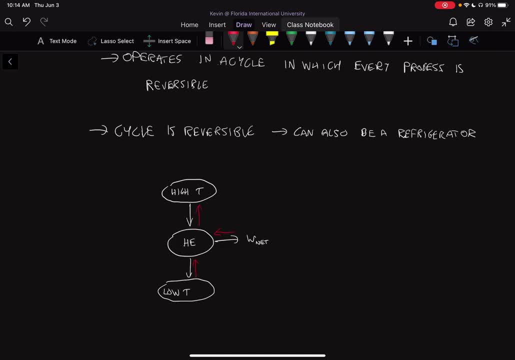 instead heat coming in from low temperature to high temperature, and that would be what we would have for our refrigerator. so our refrigerator could be reversed completely, so we can have a car- no heat engine or a car- no refrigerator, and they're just the complete opposite to each other. and in our process, since we remember, in our heat engine we 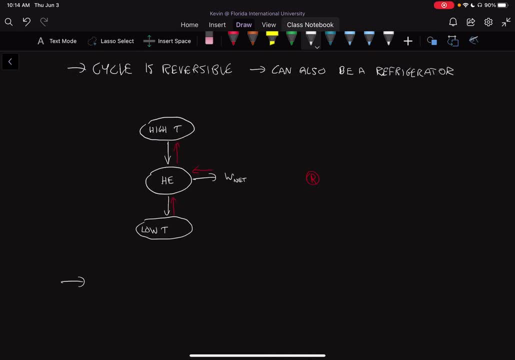 have four different uh elements, namely the boiler, the turbine, the condenser and the pump. it means that we're actually going to be seeing four reversible processes and and no heat and no friction and no losses of heat. and that occurs by having isothermal processes, where there's no change in temperature, and two adiabatic processes, which means that there's no. 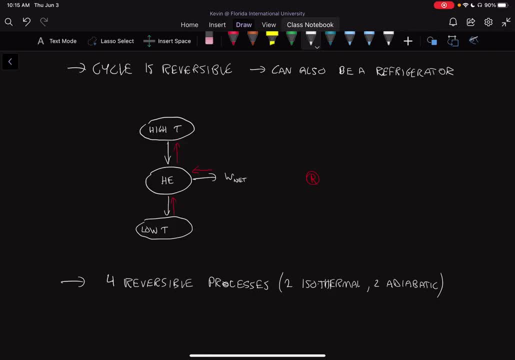 heat transfer. okay, so adiabatic means that q is equal to zero in a certain process. so let's now draw a diagram for our, for our steam power plant. so let's take an example of a steam power plant and we're going to have a steam power plant and we're going to have a steam power plant. 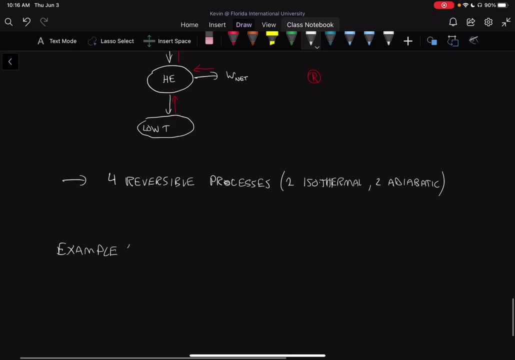 and let's work through. and let's work through what it would actually look like in terms of our car- no car, no heat engine, or car, no power plant- and how we can simplify our problem to have four reversible systems for reversible processes. so we're going to look at a power plant. 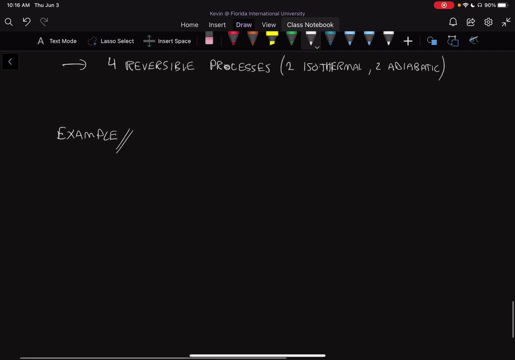 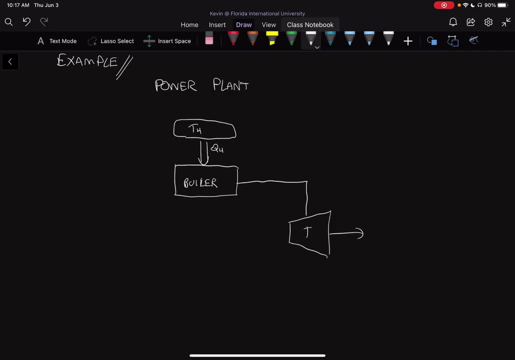 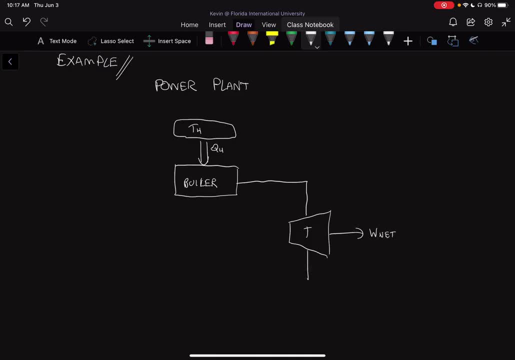 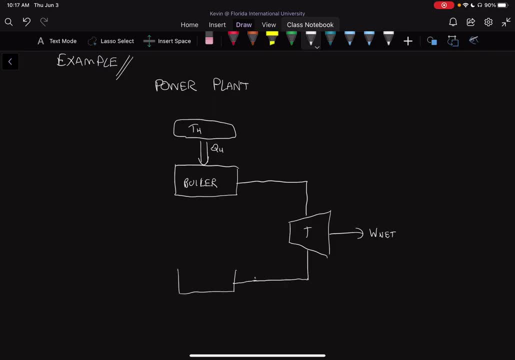 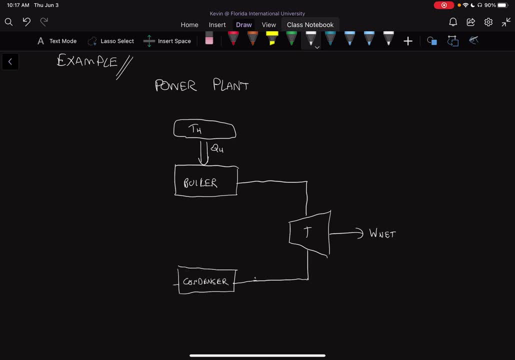 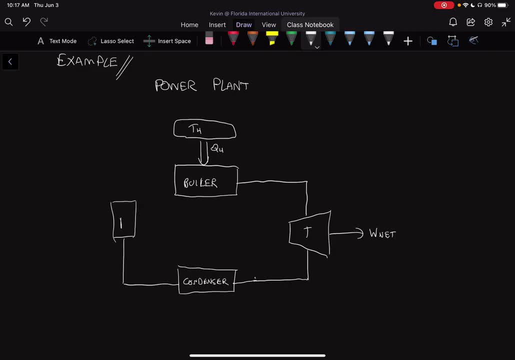 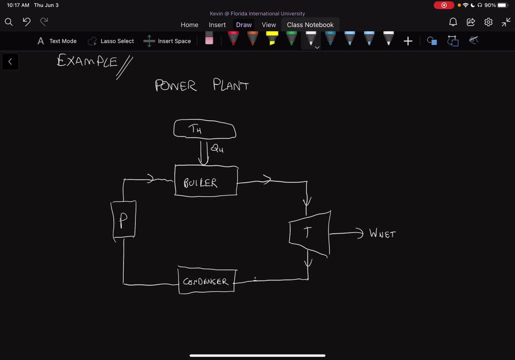 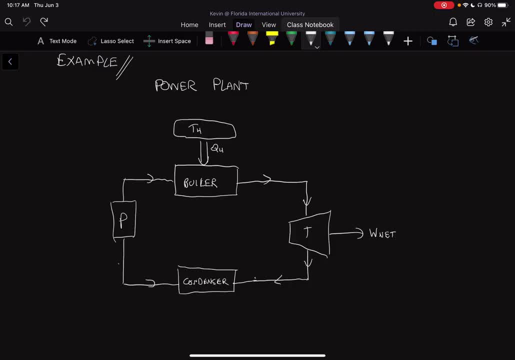 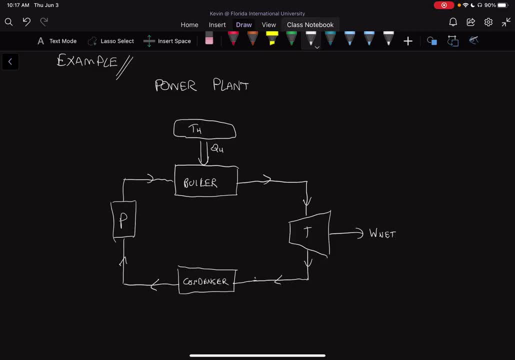 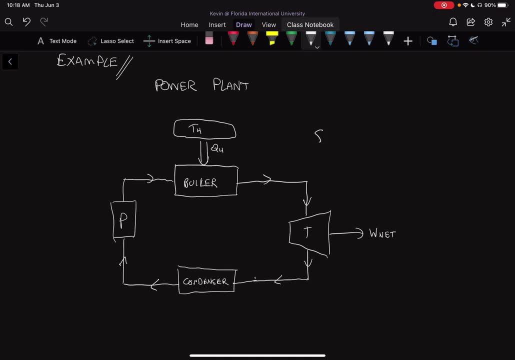 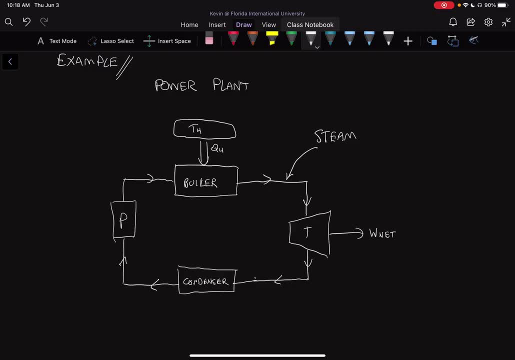 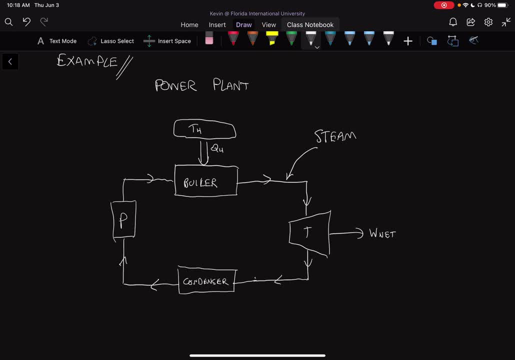 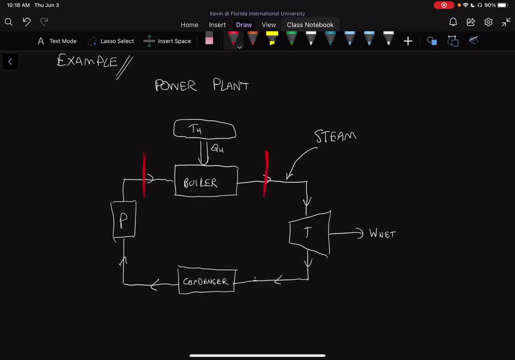 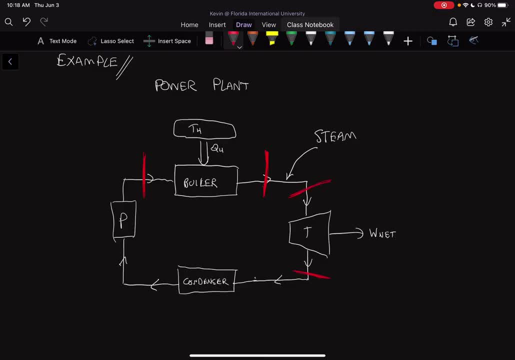 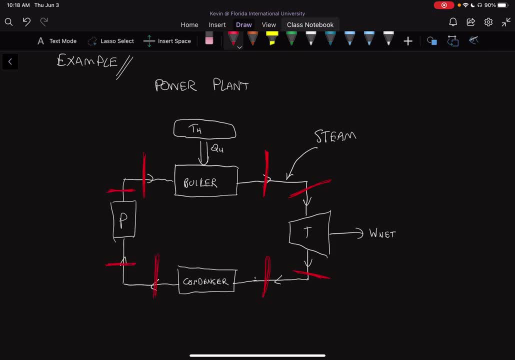 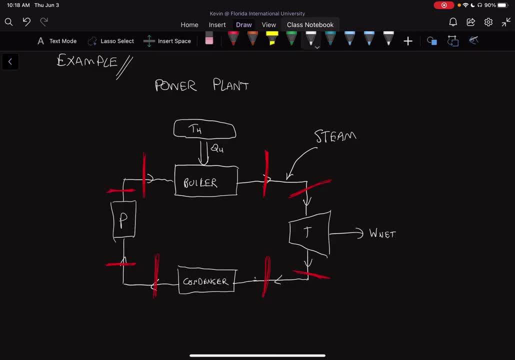 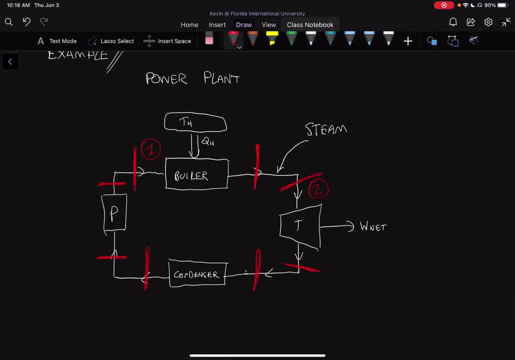 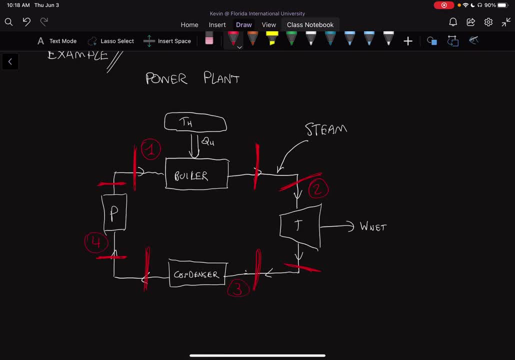 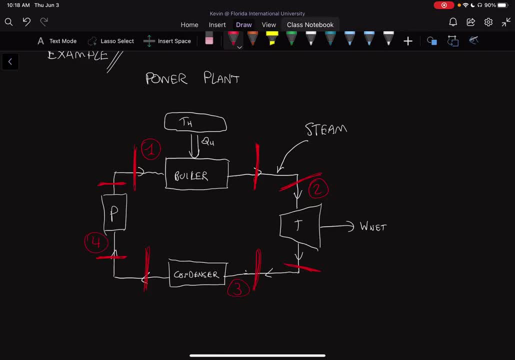 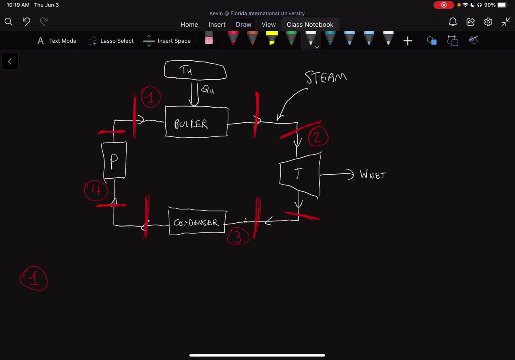 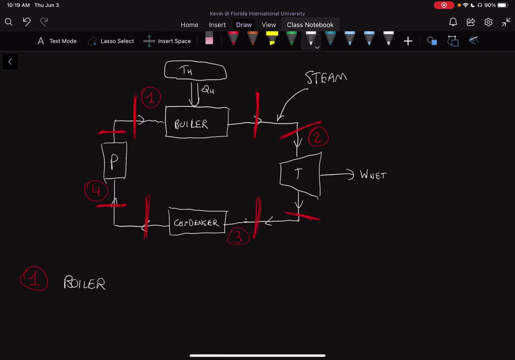 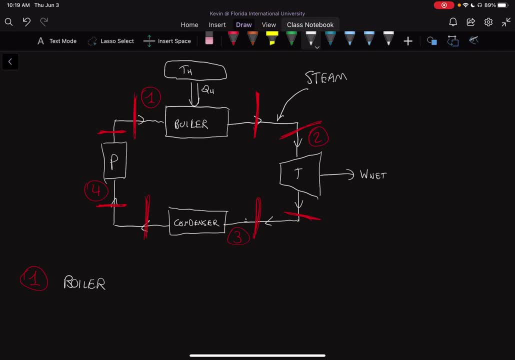 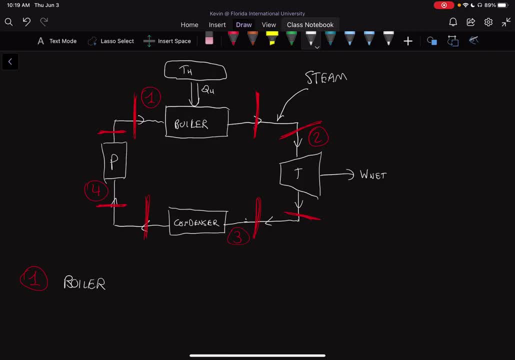 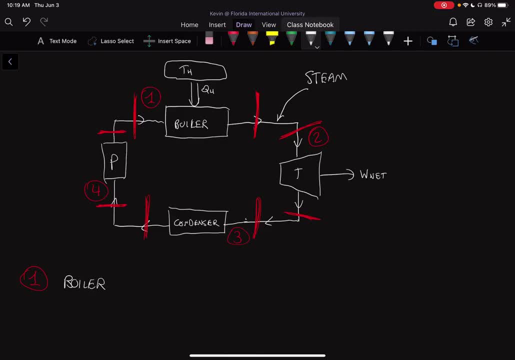 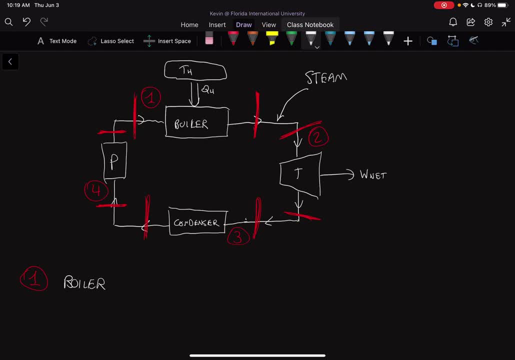 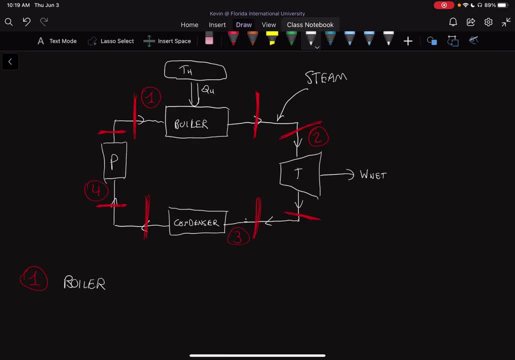 in order for our system to be ideal, what we're going to do is we're actually going to estimate what our boiler would do and we would say that heat is transferred from th and, And we can say that for the process to be reversible. so, in order for the process to 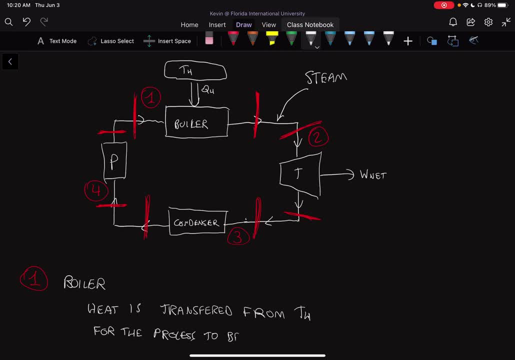 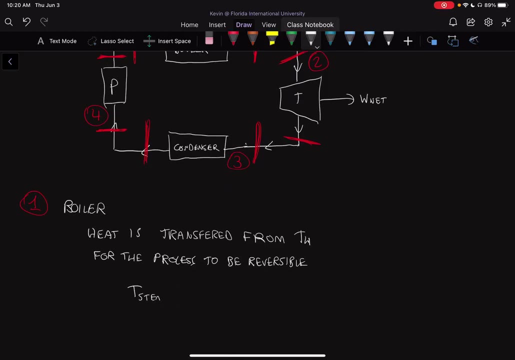 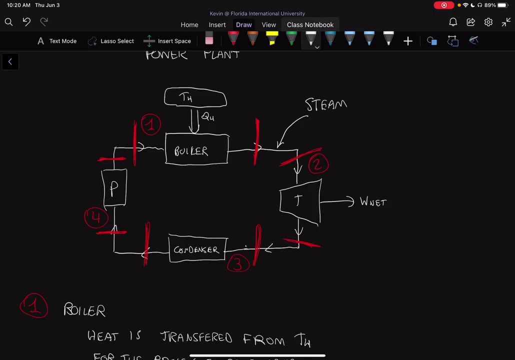 be reversible, we need the following conditions to be met: We need to have our temperature of the steam inside the tubes should be equal to TH, which is our temperature of the reservoir, and it should be constant. So, in order to reverse the process, so that the process can go either right or left in, 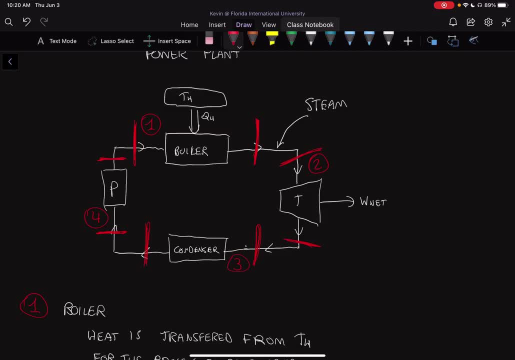 part one. we essentially need to have the same temperature here, So we need to have TH here and we need to have TH at the top, So we need to be exchanging temperature at the same exact temperature. And so what that means is that, before coming into the boiler, 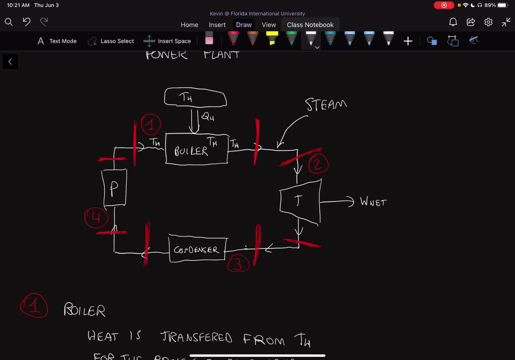 Our temperature is TH and right after coming out of the boiler our temperature is at TH And therefore our process would be one way, but could also be used the other way. We don't have any changes in temperature, So our process can be called reversible. 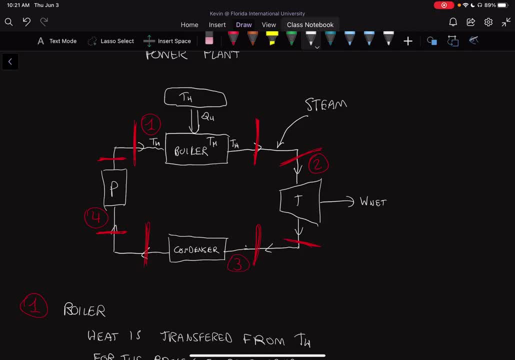 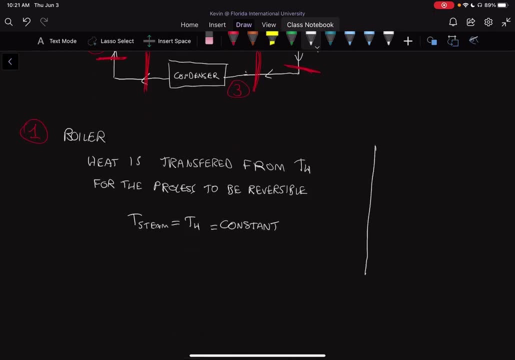 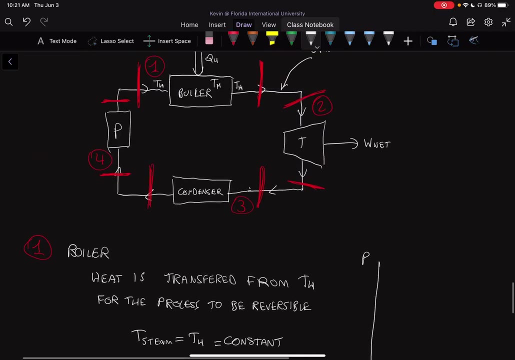 Okay, so that's the first step. Now, if we draw a p-v diagram of what is happening, We can actually draw What the p-v diagram of our process would look like. So our point one is: before the boiler and after the boiler. 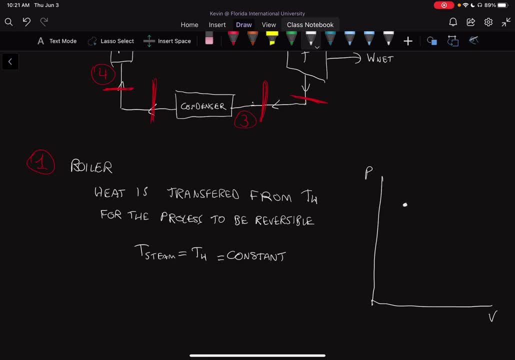 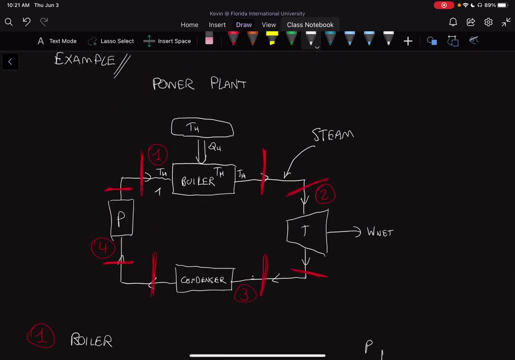 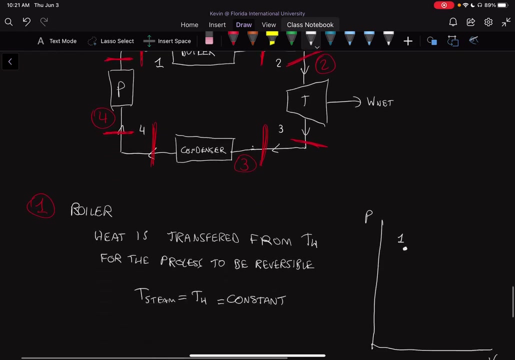 From before to after the boiler. So we'll call this little point one, Okay. so we'll do another little thing where we have point one, point two, point three and point four, Okay. So not in circles, Just little points within our system. 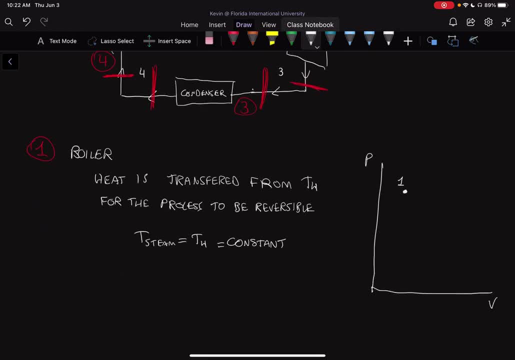 So point one would go through our boiler and would create this line from one to two, Which is after our boiler, And through here we would have some heat transfer from our boiler And this would be process number one. Okay, And we also know that during this process, 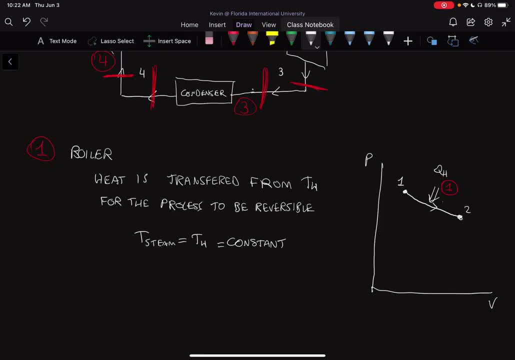 Okay, So during this process we have that th. So from one to two We have th is equal to a constant, So we know that we have a constant temperature as we go from one to two. Okay, Now number two. Let's look at process number two. 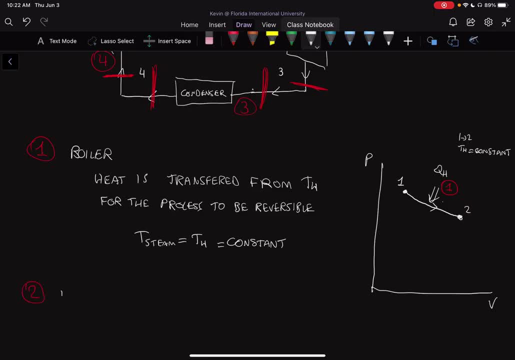 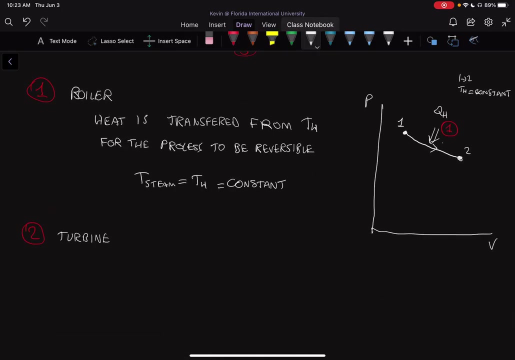 Process. number two in red is our turbine. So our turbine. We can say that our turbine is going to be an idealized system in the way that it's actually going to create some work and it's going to be adiabatic, So it's going to have no heat transfer. 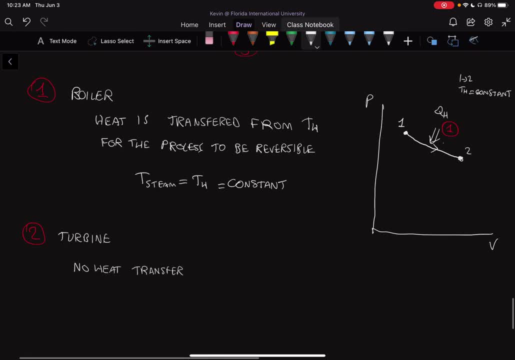 So it's as if the turbine was a perfectly isolated system with no friction and creating no heat transfer outside of it. Again, This is not realistic, But it is our goal. essentially, Our goal is to get the most perfect turbine so that all the fluid coming in and going. 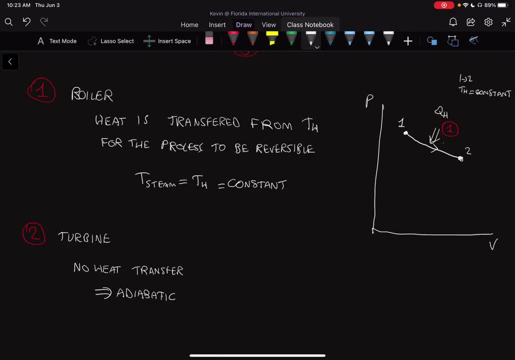 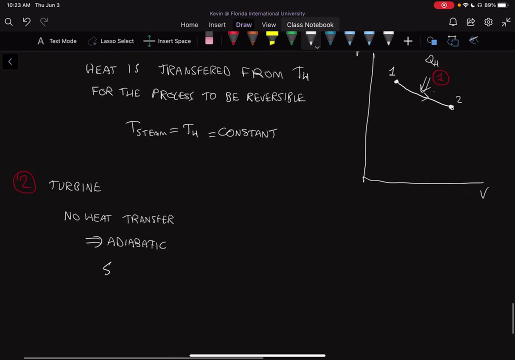 from a high temperature to a low temperature creates some work out of high temperature to low temperature. So we can say that in the turbine steam has to go From th To t L, So it has to go from a high temperature to a low temperature. 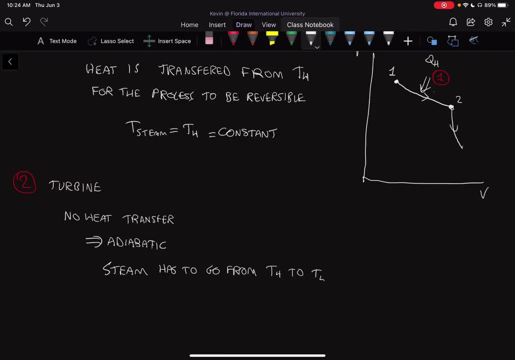 And in our process diagram it would look something like this: So we would go from two to three And we would now jump from th To t L, Essentially Okay. So we would go from th to t L, And we know that from two to three we would have q. 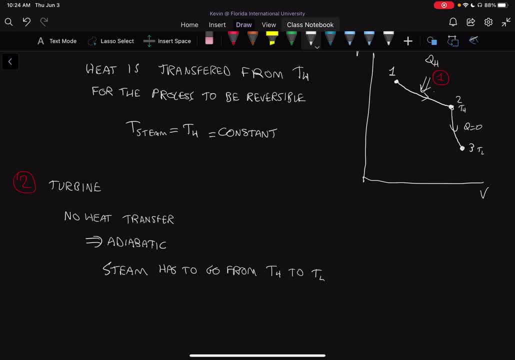 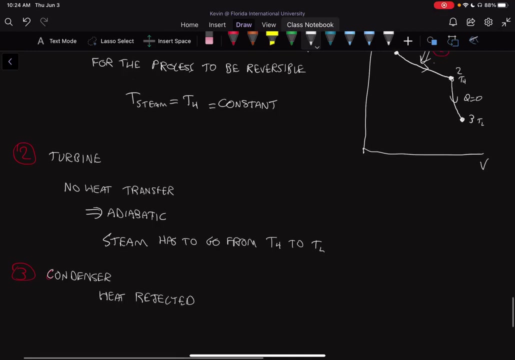 Is equal to zero, So we have no change Process. number three is for our condenser. In our condenser we essentially have heat being rejected, And this heat is going to be rejected at constant temperature of t L, So it's going to be at t. 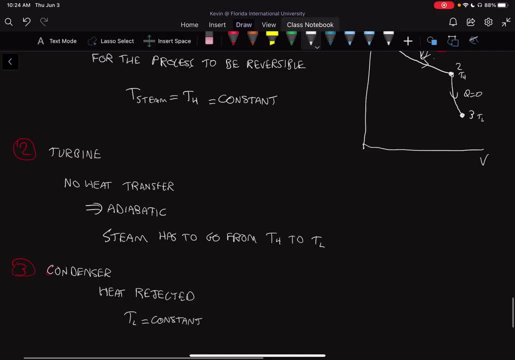 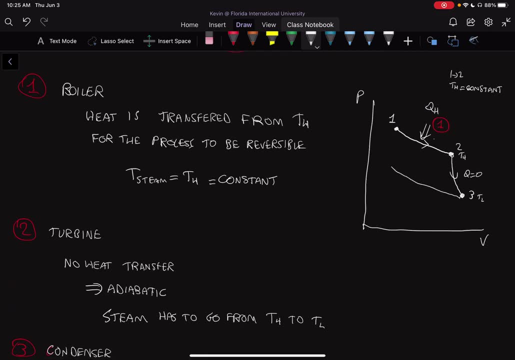 L Is equal to a constant. Okay, So We're going to have some heat rejected And this process is going to look something like this, And we're going to have some q L Out, And so, from three to four, we're actually going to have a constant t. 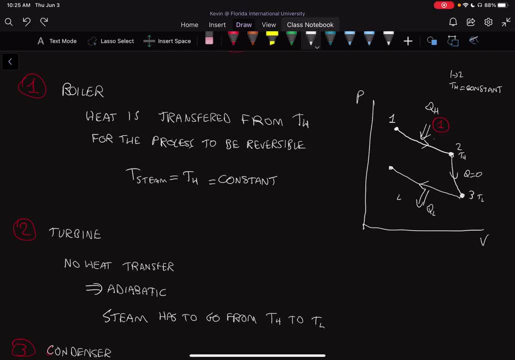 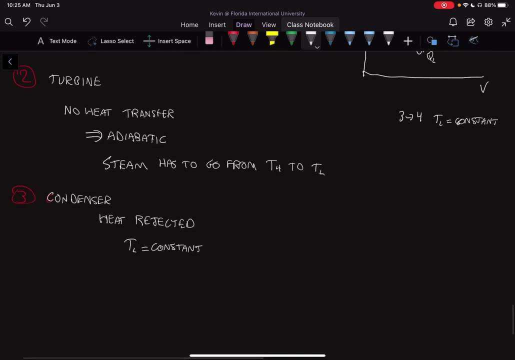 L, So from three- sorry, let me put four in the right spot- So from three to four, we're going to have t. L Is equal to constant, And then, finally, our pump is going to bring back by increasing the pressure of our fluid. 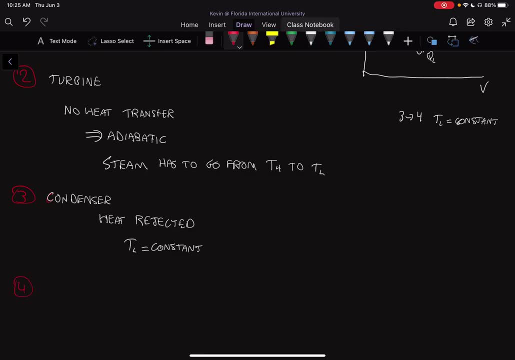 Our pump is going to bring back our t L Back to th, So we have an adiabatic process. So it's the pump, We have an adiabatic process. Bring T L To th And we bring t. 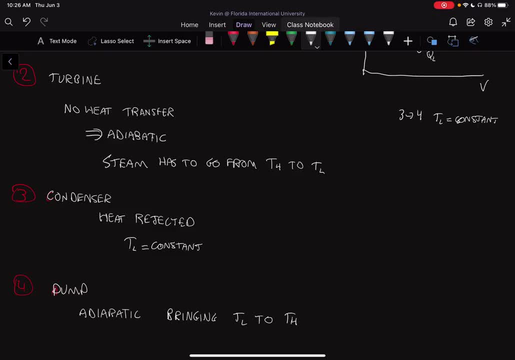 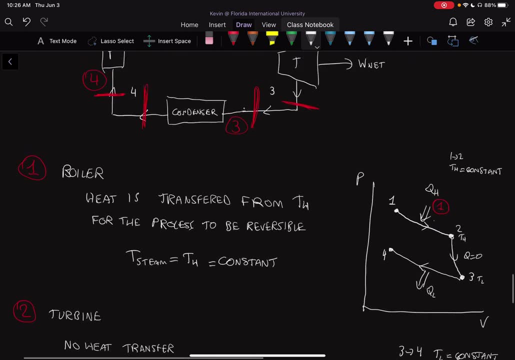 L To th By essentially compressing the fluid. If we add pressure and we keep the volume flow rate the same, we're going to increase our temperature for our system, And so we have a final process that looks something like this, And it's a little curved. 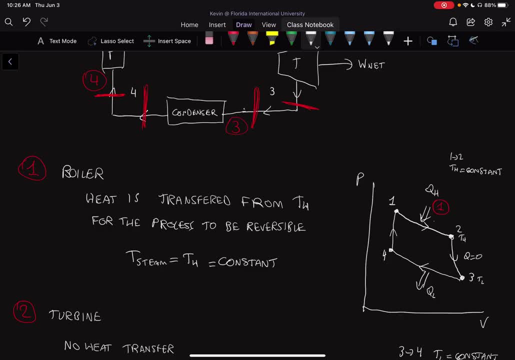 It's not a straight line up, But Just Let me try to bear with me. So It would actually look something like this. So let me just redraw it so that it's perfect. We would have three to point four And then point four to point one, like this: 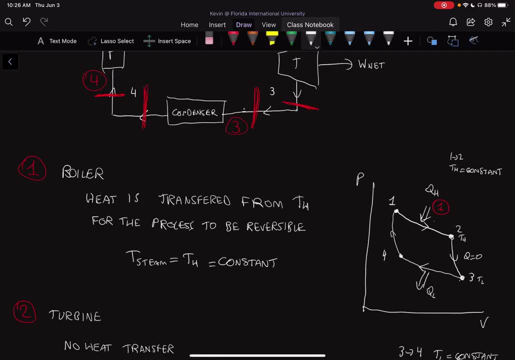 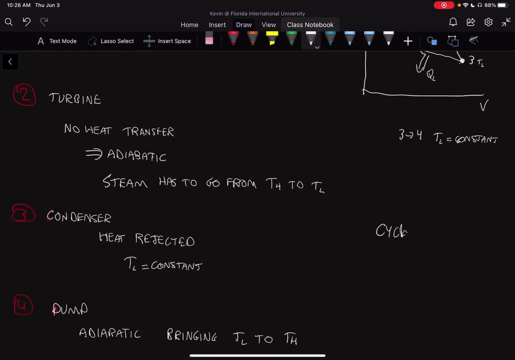 Okay, So that all curves are curved and not just straight lines, And this whole cycle Is reversible. So since it's for reversible process, The cycle Is also reversible. Okay, That's very important to note. And, once again, The pump here. 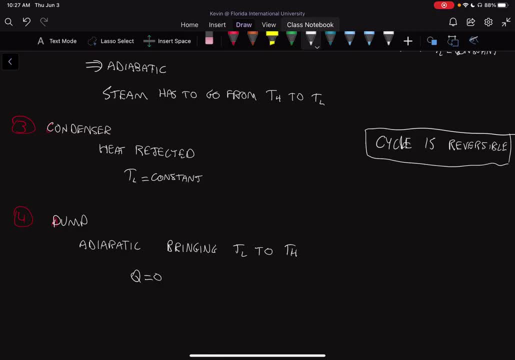 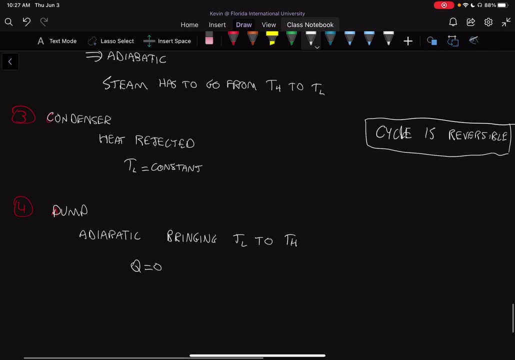 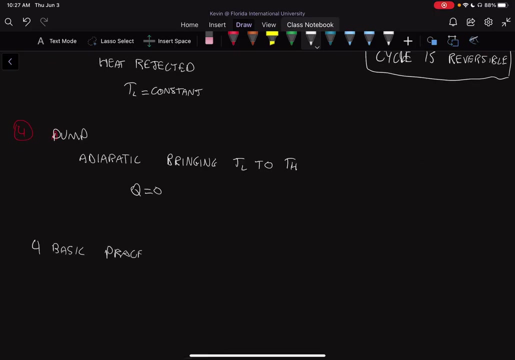 Q is equal to zero. Okay, Just making sure that we understand this. Now, If we Summarize the processes And the four basic processes for our system, Okay, So We have One, What is called a reversible isothermal expansion. 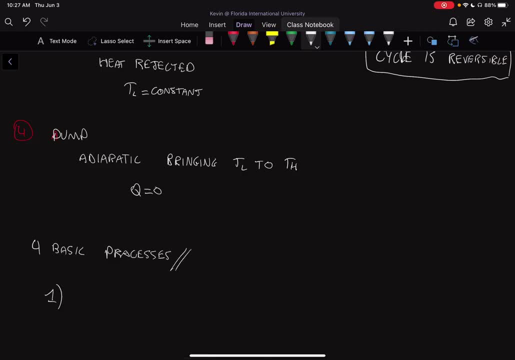 So we have a reversible Rev. I saw thermal Expansion. Okay, And this isothermal expansion happens with our Q H In our boiler And we have a new, So One What is called a reversible isothermal expansion. 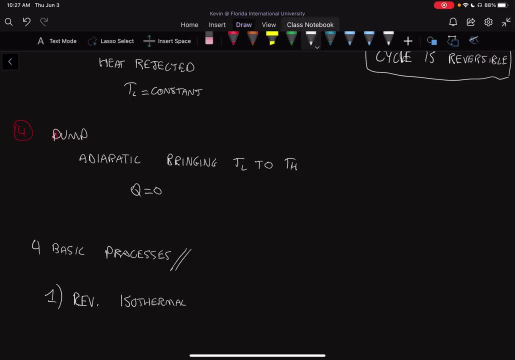 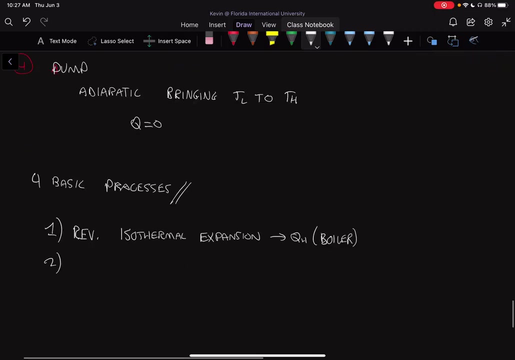 Okay, And this isothermal expansion Happens With our Q H In our boiler. Okay, So that's been the first step And we have A reversible Rev Isothermal Expansion number two. we then have a reversible adiabatic expansion as well. i'll put exp for expansion. 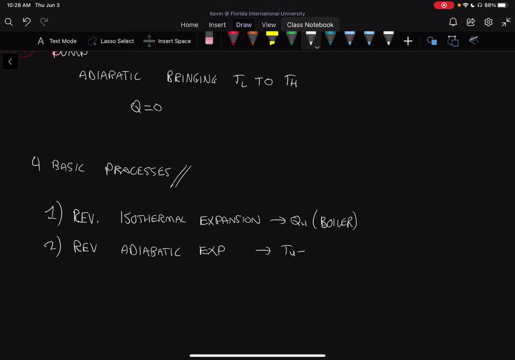 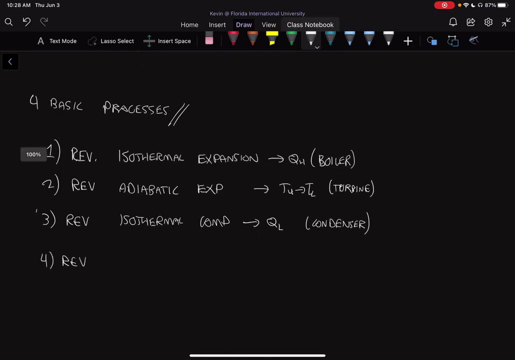 just to keep it short. where we go from th to tl in our turbine, then we have a reversible isothermal compression, and this compression happens at ql and this happens in the condenser. following that, we have a reversible adiabatic compression which brings tl back to th, and this happens in our pump. 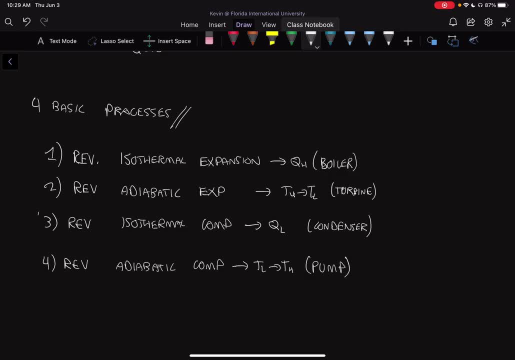 okay, so we've described what a carno cycle would look like and the particularity of the carno cycle is that we have isothermal systems and adiabatic systems in our process. in real life we don't have adiabatic and we don't have isothermal expansion, so in real life we don't have those exactitudes and those. 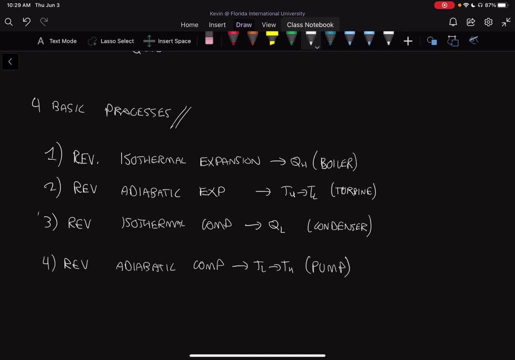 perfect systems. okay, so, moving forward from this, let's talk about the thermodynamic temperature scale and explain a little bit of how we can use our carno cycle, our carno system, to simplify our analysis of these problems. so we're going to look at the thermodynamic temperature scale. 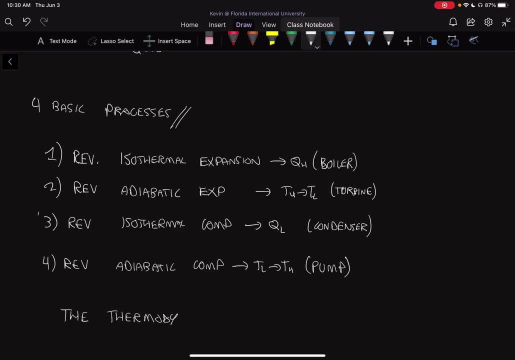 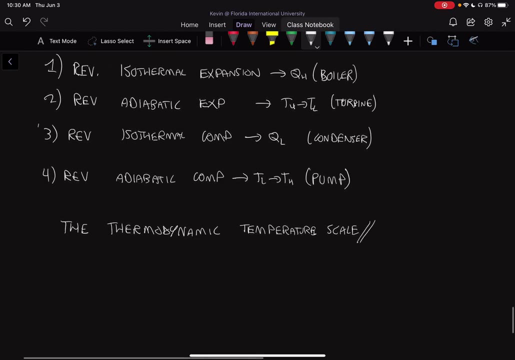 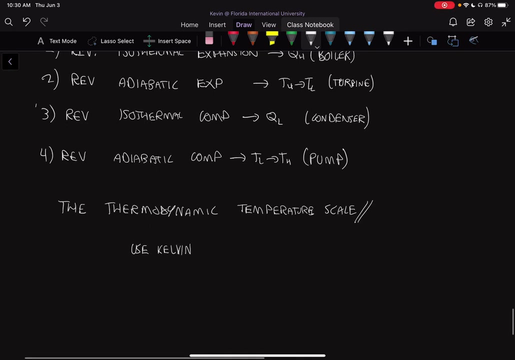 so we can say that in thermodynamic temperature scale we can have a temperature scale that is equal to the thermal efficiency of the cycle and we have to use kelvin always. and let's look at how we're going to be able to use our kelvin, our absolute temperature. 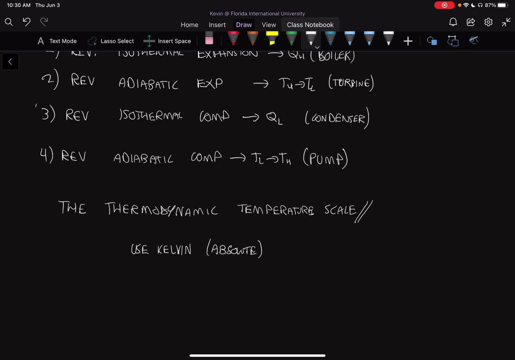 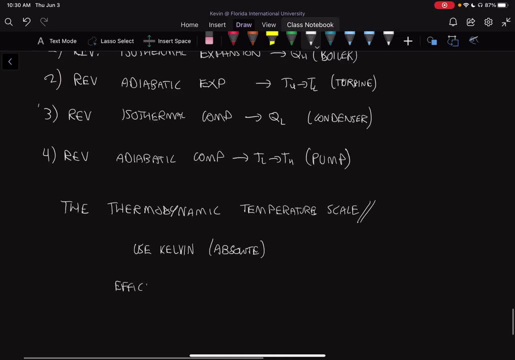 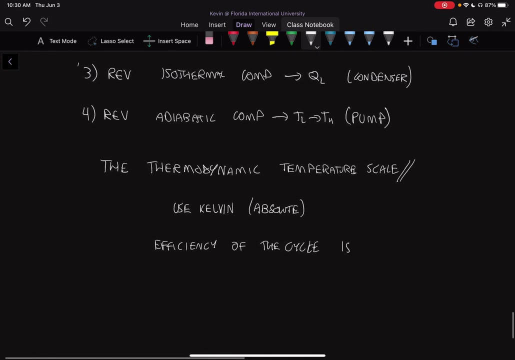 within this system to analyze it. so the first thing we can say is that the efficiency of a cycle, so the efficiency of the cycle, the thermal efficiency of the cycle is, we can say it is a function of what. So we have thermal efficiency is equal to a function of QL and QH right. 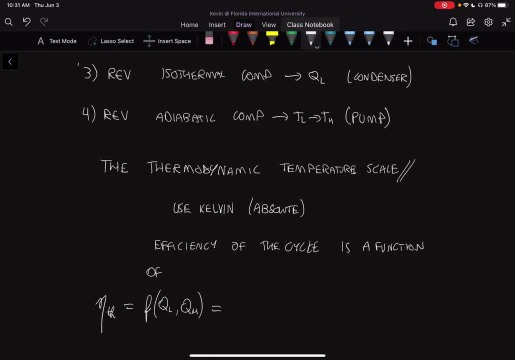 If we look at the equation for thermal efficiency, we have that thermal efficiency is equal to work net over QH. So it could be a function of work net and QH. But we also wrote that it can be just a function of QL and QH. 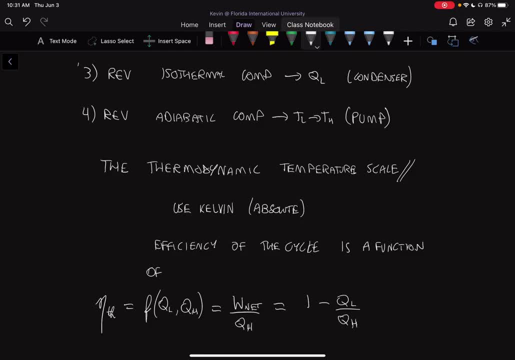 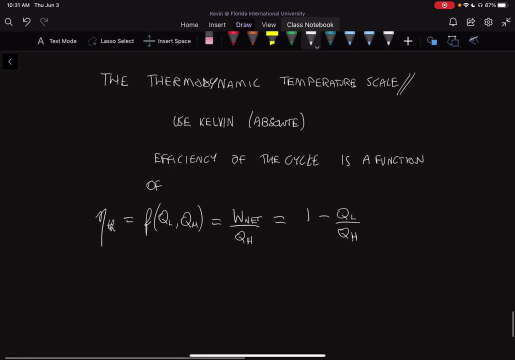 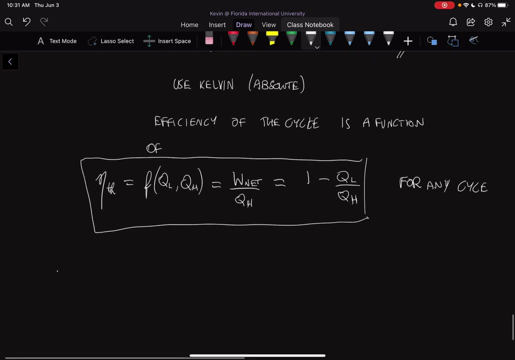 if we substitute for work, net is equal to QH minus QL. Okay, that's for any cycle. Okay, so for any cycle we can say this is true. Now, in a Carnot engine, we can make some further assumptions. 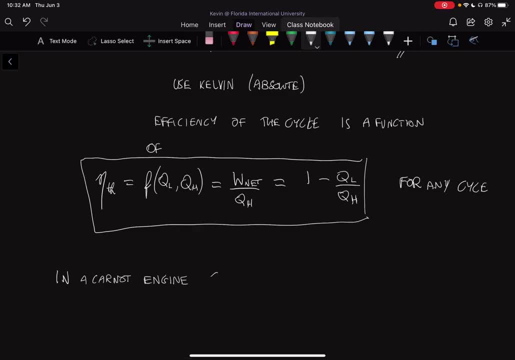 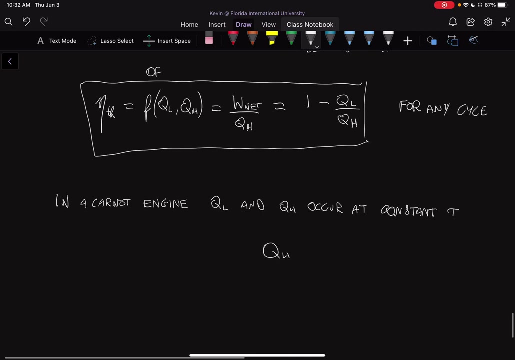 We know, in a Carnot engine QL and QH occur At constant temperature. So in this ideal engine we have, QH and QL happen at constant temperature. Now that means that if we have a constant temperature we can rewrite QH and QL as our heat transfer is equal to mass times, CP times, TH. 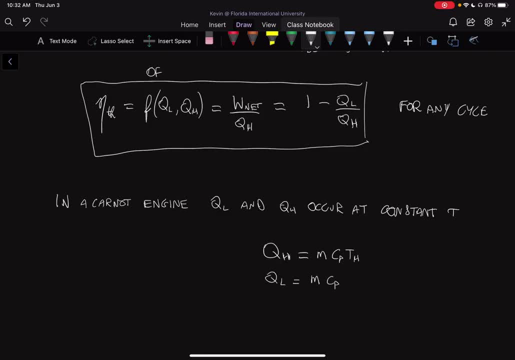 And QL is equal to mass times, CP times, TL. That would be the equation for our heat transfer And we can see that, essentially, TH is directly proportional to QH and TL is directly proportional to QL. This is only true if the temperature is constant. 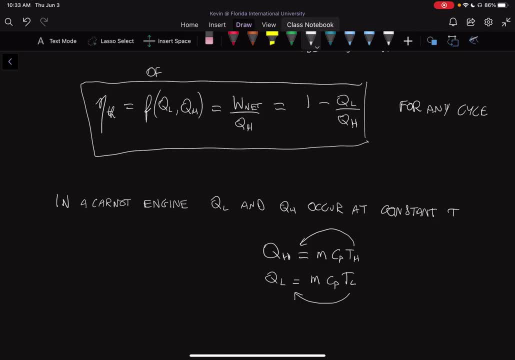 If you have a change in temperature in your system, your QH is not that equation, It's more complicated. Okay, you then have to look at your change in, you have to look at your change in temperature within your system, and it makes it more complicated. 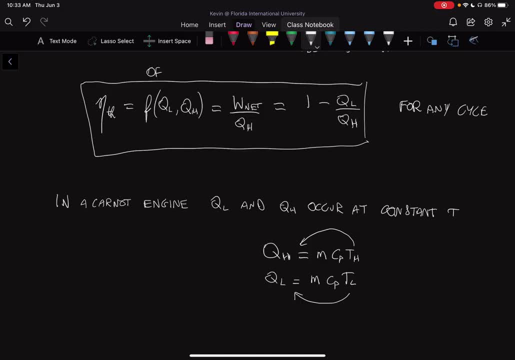 But what that means for a constant temperature system or an isothermal process is that we can say that the N thermal for Carnot- so only for Carnot- is equal to another function of TH and TL. So we can say that the thermal efficiency. 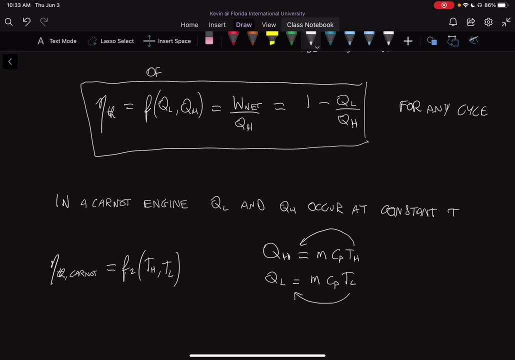 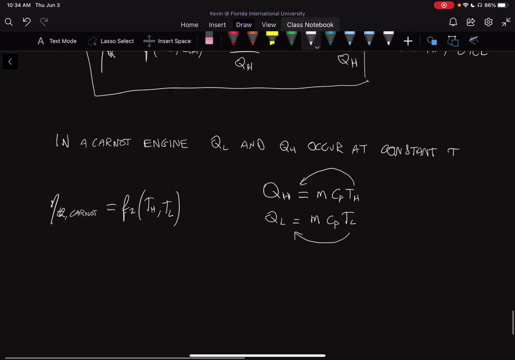 since temperature is directly related to QH and QL, we can say that the thermal efficiency is equal to a function of the temperatures. now, Okay, And for Carnot, if we actually look at what QH over QL would be, QH over QL would happen to be TH over TL. 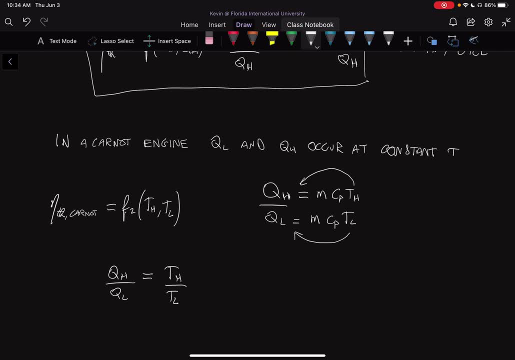 just by dividing the above equations. So if you do QH over QL, you have MCP, TH over MCP, TL, MCP cancels out and you're left with TH over TL. And again you have to make some assumptions here that CP does not change. but we assume that CP is pretty much. 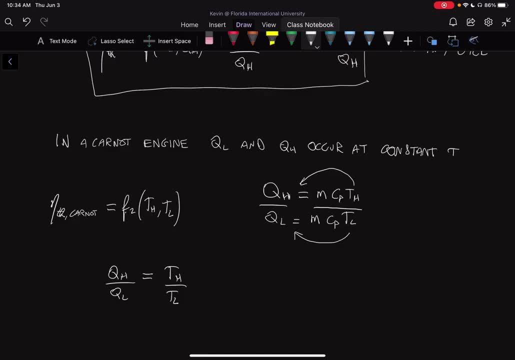 the same. we assume that M is the same. So we have that QH over QL is equal to TH over TL, And this is for Carnot only. Okay, so we have to make sure that we use this only for Carnot. 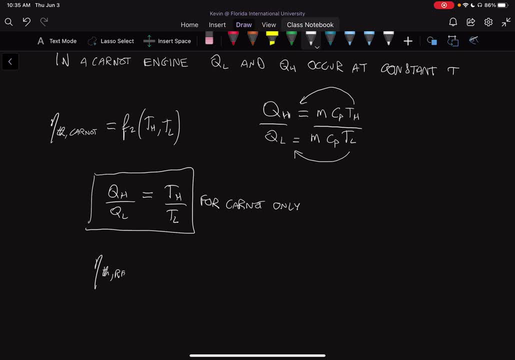 So that means that the N thermal of a reversible system, or REV, is equal to the N thermal of Carnot. So you're free to use whichever you want. Reversible or Carnot is the same thing. And that is equal to one minus QL over QH. 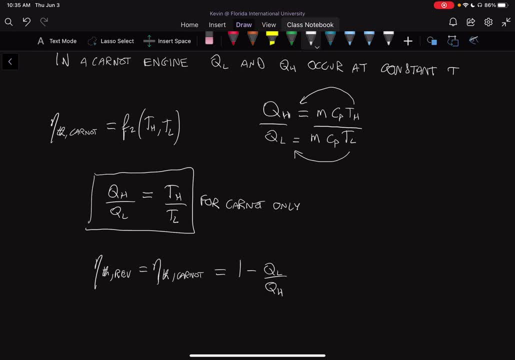 So that still holds right. This is our for any cycle. we know that thermal efficiency is one minus QL over QH, but now, with the Carnot engine, we can write this equation as one minus TL over TH. So what that means is that if we have, you know. 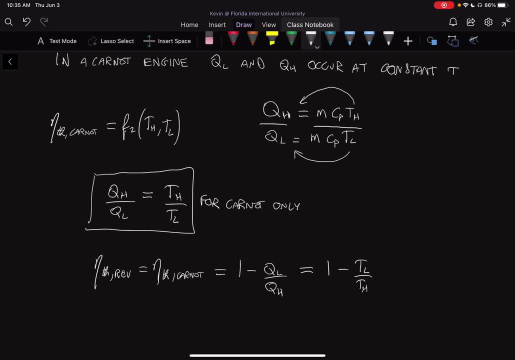 if we have one minus QL over QH, we can write this equation as one minus TL over TH. So what that means is that if we have, you know, a steam power plant and we're trying to find the Carnot efficiency or the efficiency, 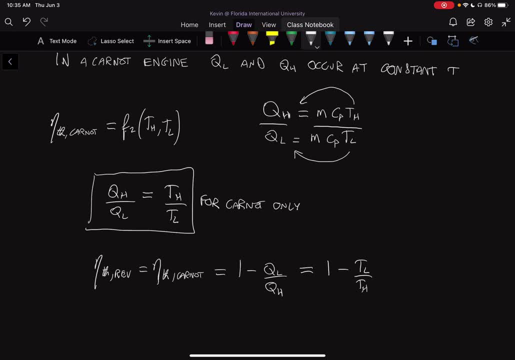 of if the steam power plant was designed as a Carnot. we could literally just say that if we know the temperature of the high temperature reservoir and the temperature of the low temperature reservoir, we can find the thermal efficiency or the maximum thermal efficiency of our heat engine. 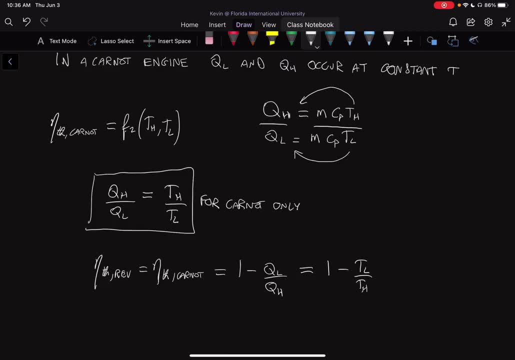 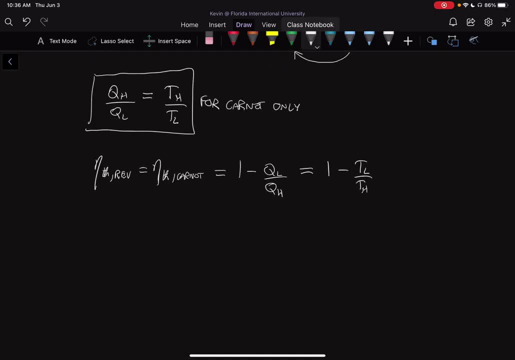 Okay, So a little bit of description as to how we describe the three types of engines that we can see, or the two types of engines that we can see, is an irreversible system will always have N. thermal is equal to one minus QL over QH. 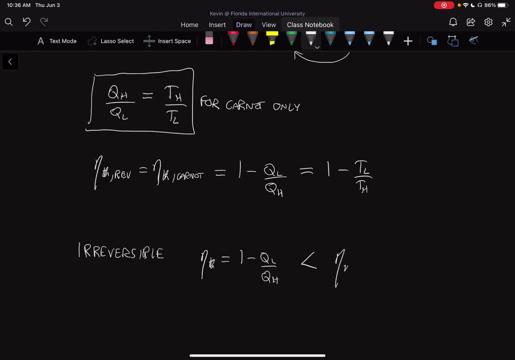 and will always be less than or equal to N thermal reversible. Okay, A reversible heat engine will have N thermal is equal to N thermal reversible. So it's equal to a reversible system. It makes sense. Okay, This is to describe so. if we know that we have, our thermal efficiency is equal to the reversible thermal efficiency. we therefore have a reversible heat engine. 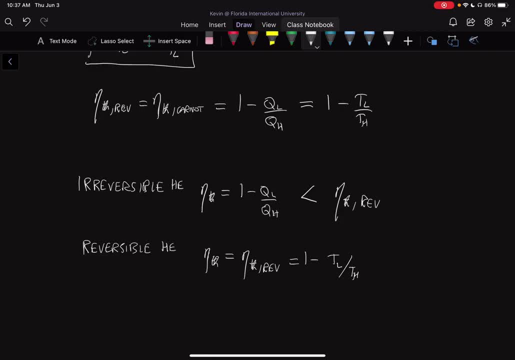 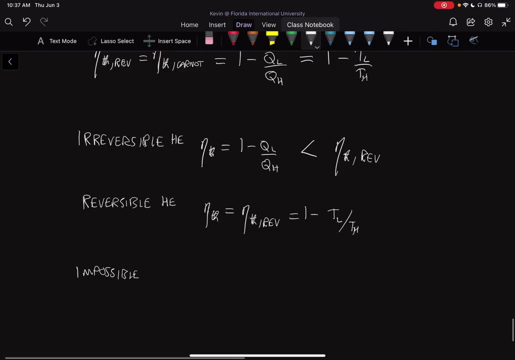 Okay, makes sense, And I'll just add HE here. so we know we're talking about heat engine. Now an impossible heat engine, which is our third type, would be a heat engine that we design and we say: okay, we find out that after designing it and after doing simulations, for example, we have N thermal is greater than N thermal reversible. 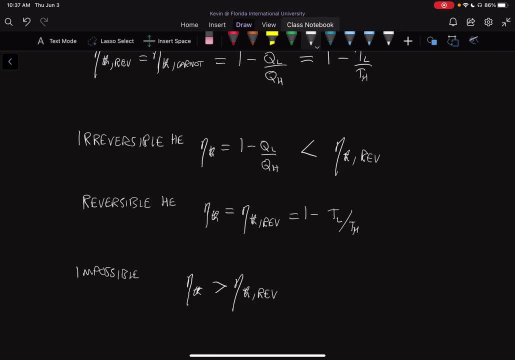 This is impossible to happen. Okay, it can happen if we make up numbers, but it's impossible for it to happen. Now let me show you why we cannot have a steam power plant have 100% thermal efficiency. Okay, so the reason why we can't have 100% thermal efficiency is for the following: 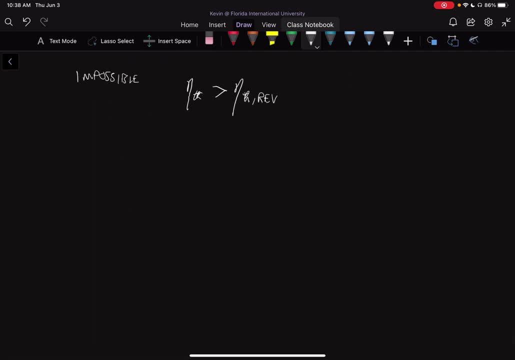 Let's look at a perfect steam power plant that operates between two temperatures, and this perfect system is reversible and operates under a Carnot cycle. So we have a steam power plant. It operates between 1,000 Kelvin- so that's our hot side- and 300 Kelvin- okay, which is usually our temperature in our environment. let's say: 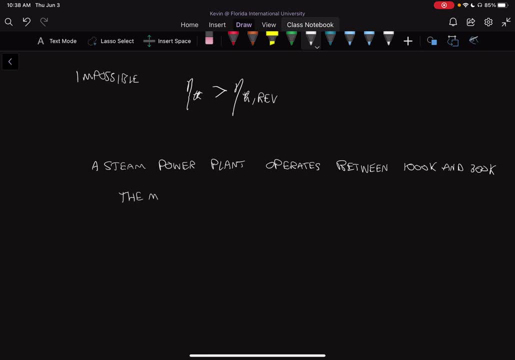 Well, the maximum thermal efficiency is going to be equal to the thermal efficiency. So what we're going to do is we're going to plug in our values of our reversible, And so that means that it's going to be NTH. rev is 1 minus TL over TH. 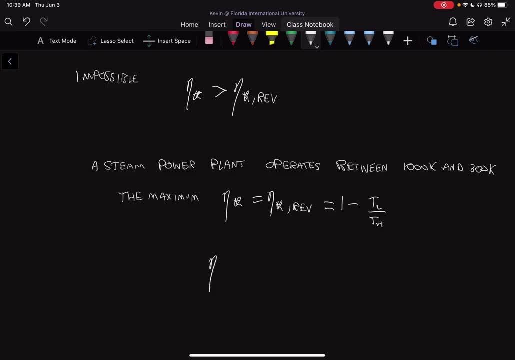 And if we plug in our values, we get that N thermal reversible is equal to 1 minus 300 over 1,000. So we get that this is equal To 70%. so our theoretical maximum is actually 70%. okay, so we see that the only way for us to get a theoretical maximum very, very close to 70% would be to essentially dump out our system at 1 Kelvin or something like that, or 2 Kelvin, but that's very, very unlikely, on this earth at least. 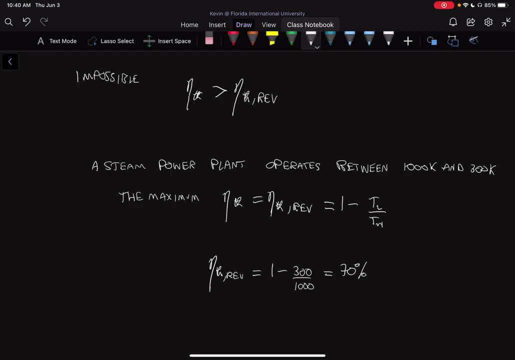 Okay, so we're never Really close to 100%. Now the other way we can do it is increase TH. So if we increase TH to 100,000 Kelvin, then we're able to get our thermal efficiency as high as possible. 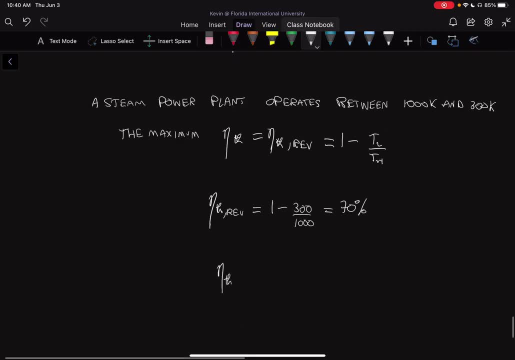 A typical thermal efficiency. a regular thermal efficiency for a power plant is around 40%. So you can see that we're pretty far from the 70% max. Now how do we maximize efficiency Of a heat engine? to maximize the efficiency of a heat engine? reversible or not really, because they both would increase. 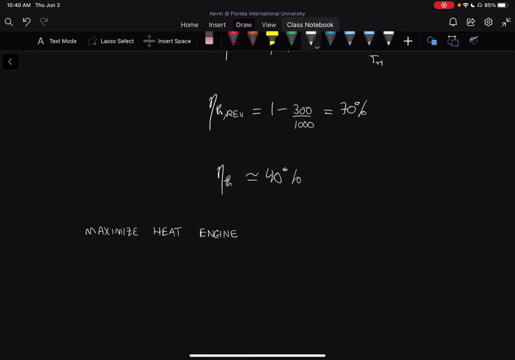 So if the reversible limit increases, usually your thermal efficiency for your actual system also increases. but essentially what we want to do to maximize the heat engine efficiency is the following: We want to increase TH, so we want to have a hotter TH and we want to have a cooler TL. just from our equation. 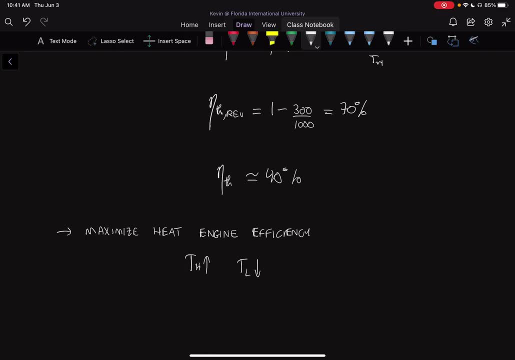 Okay, we want to be able to do that so that we get a better thermal efficiency. Okay, now the refrigerators and heat pumps work in the exact same way, So we can use the equation for Carnot Refrigerator, since they all use the same processes. just reversed the Carnot refrigerator plus heat pump, and remember that the heat pump and the refrigerator are the same system. the only difference is the goal changes. 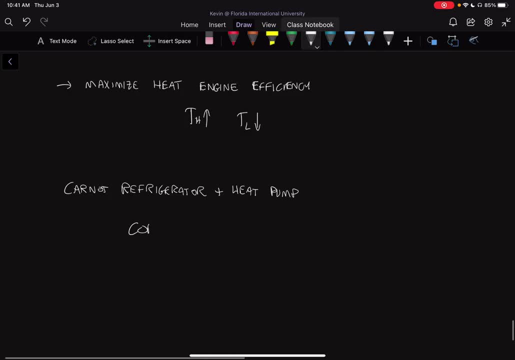 So our coefficient of performance for our refrigerator- reversible- would now be equal to 1 over TH, TH over TL minus 1, and the coefficient of performance of our heat pump- reversible because the goal is different- would now be equal to 1 over 1 minus TL over TH. 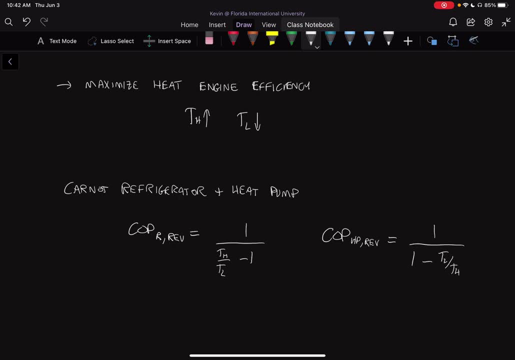 Okay, so we're going to take a break here and in the following part of our lecture we are going to be looking at two different example- problems using Carnot and trying to understand Carnot- and that will conclude our module 5 for this class. 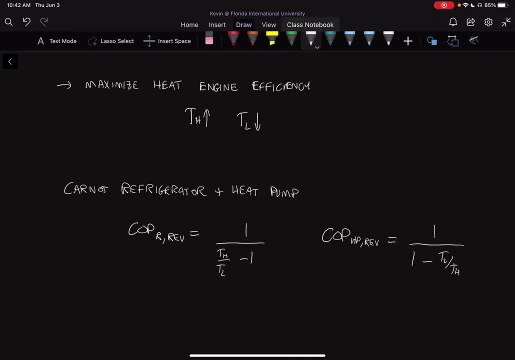 So we'll see you in the last part of module 5 for two example problems from your book.